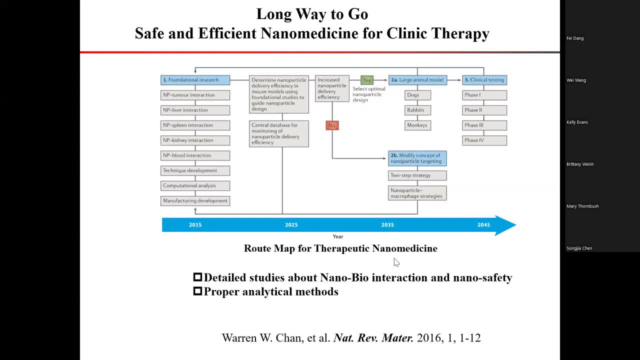 From this roadmap for therapy nanomedicine. we still need 30 years to go to obtain an excellent nanomedicine. We can see that we need to know many information about how nanomaterials interact with our tissues, such as with tumor, liver, spleen, kidney blood and other system. 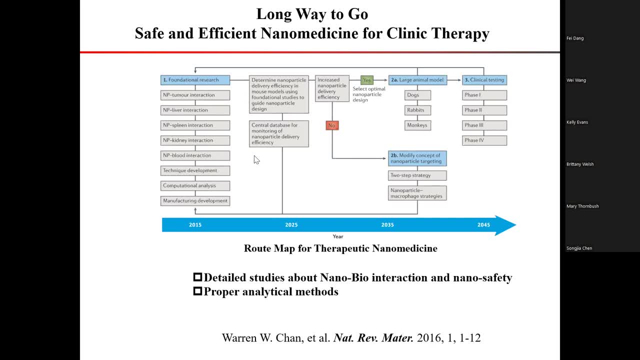 Next, we need to know how nanomaterials interact with our tissue. Next, we need to know how nanomaterials interact with our tissue. Next, we need to know how nanomaterials interact with our tissue. If nanomaterials interact with small animals and larger animals, then we need to, based on this information, modulate the properties of nanomedicine to have good performance and also good safeties. 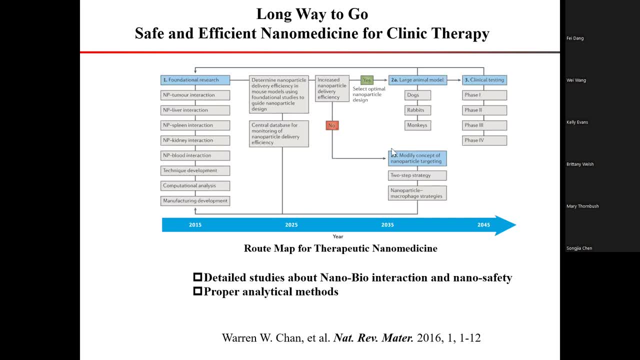 That takes a long time During the study. we should take some powerful analytics. During the study. we should take some powerful analytics method to study how they're in the room at the different levels and then know the important knowledge is at the 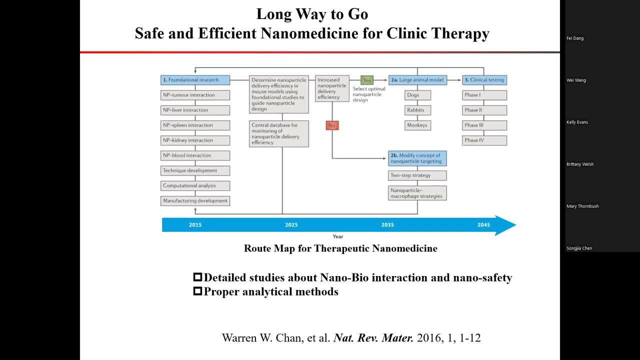 different levels, then when you, based on this knowledge to design the nanomedicine, have a good performance and productivity. So that's the reason why we need no time to to design and develop a known how to develop a good nanomedicines And other window, the balance system is very 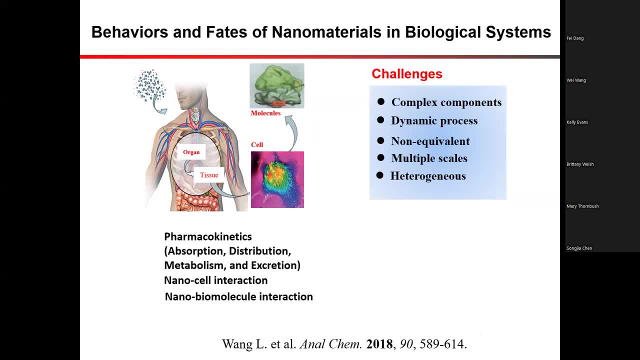 complex For the whole whole body of home being a home being. one nanomaterial is both to home being and they will be absorbed and distributed in different tissues and organs. And then some tissue organ like a navel and spleen material may. 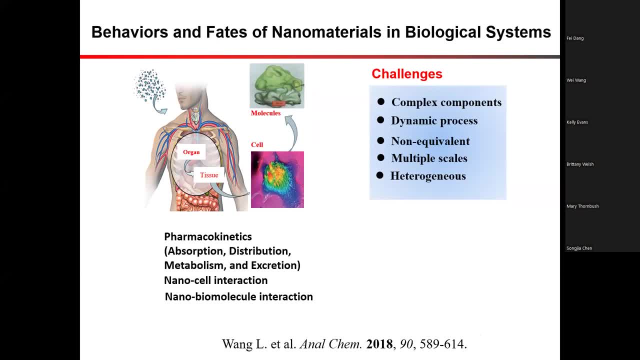 stay there for a long time, or part of them may be metabolized and and secreted by the urine and facilities. A small part may remain in the tissue for a long time. So during the interaction there are some complex reaction happened In. 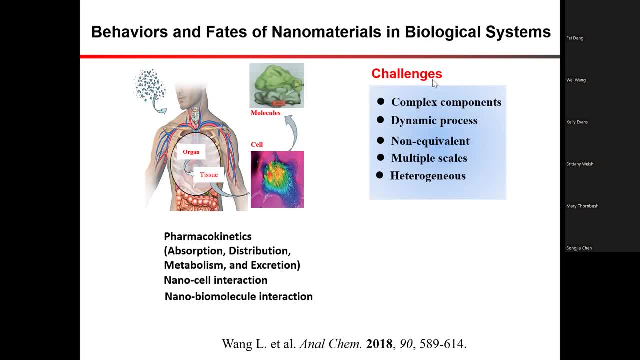 fact, due to the one reason is the complex system, the system they have. they include many kinds of molecules, cells and tissues, and the condition of proteins and the molecules, And in heterogeneous, with different condition and different distributions. Moreover, the interaction is a. 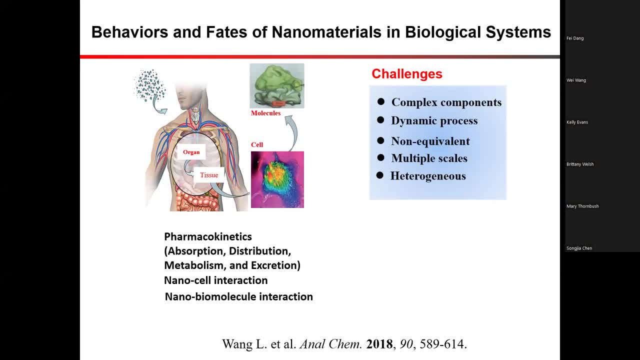 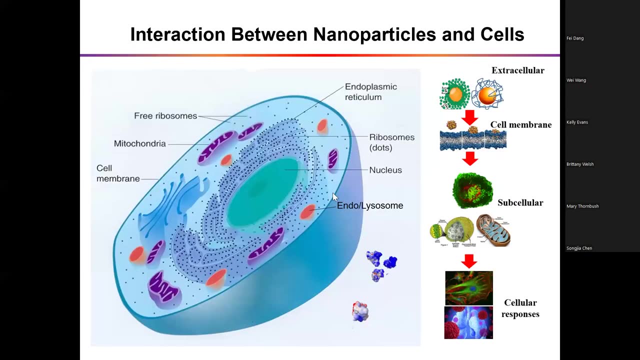 dynamic process, the one nanomaterial, interweave with cells and with the proteins. So all all the things are so complex that make the study for nano core body study very complex, Even for the simple cells. nano and cell interaction is also complex, For example when 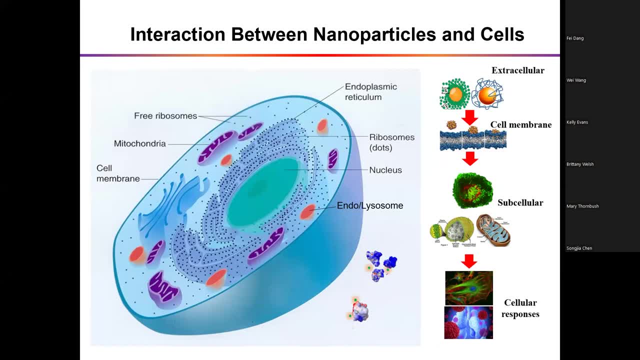 nanomaterial interweave with cells, first the, so the proteins in the environment, and they form. then they form the, some nano protein coronas on the surface. the complex may be recalculated by the cell receptors And then they try to. 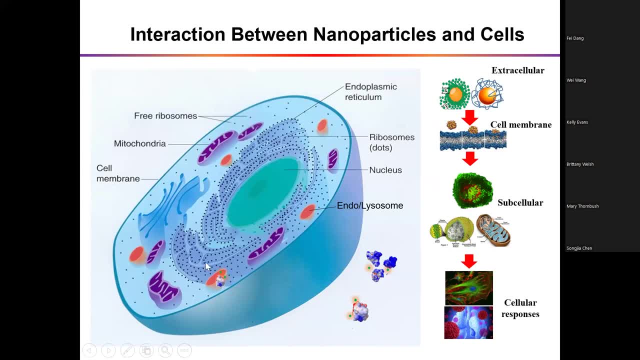 turn and turn located to the endosome and non-some In the future. we are not sure that. so there is a problem and we can actually apply the same amount of the禹. I will definitely give you some information on the differences. Okay, Okay, Thank you very much. Thank you for your time. Okay, Thank you very much. So, yes, this is. this is the後. I also mentioned when the person will be on the call. they will be on the endosome of the cell. 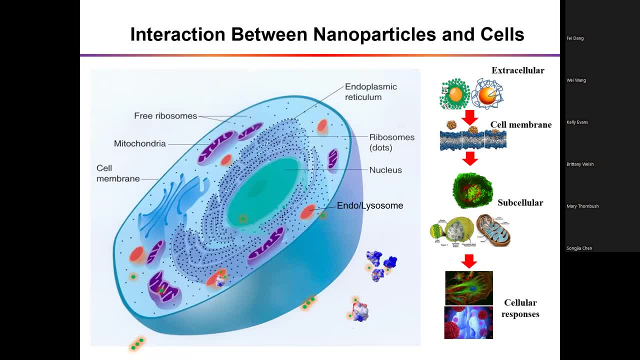 Lianfeng Zhao, PhD, And then the mature changes are liquidation and the physical and chemical conditions all the time. so if you want to know what happened to the sales during that interaction, we need that confirm. or the what happened to net materials. these are the. maybe the reason because there's some biology with both SM. 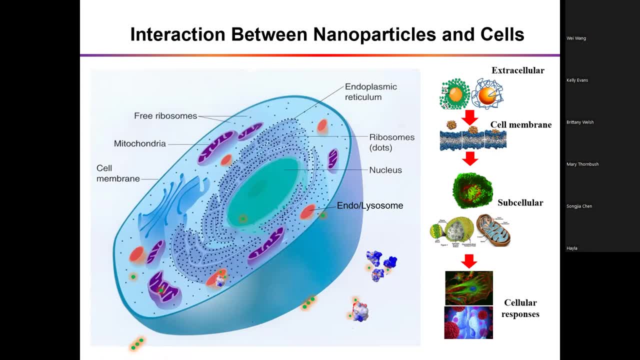 Lianfeng Zhao PhD, biology effect of of some effect. so to to know the question, we we needed to have a separate question. first of all, then, mature Intel with the environment. why is the protein? another is the Lianfeng Zhao PhD nip it. yet protein is outside of the sales. inside the sales also have an income, some proteins. so nanoprotein is the bit, because 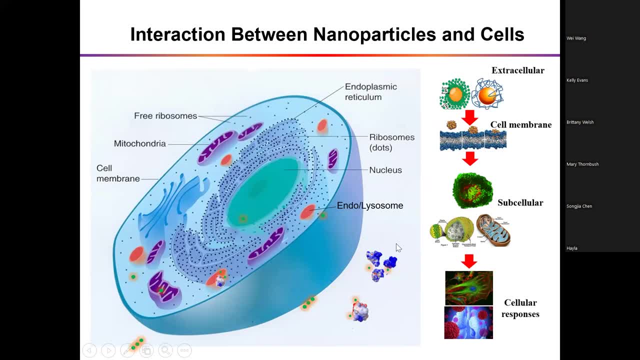 Lianfeng Zhao, PhD, An interaction during the nano bio interface. another thing: even nano nip it. when then particle is going inside sales, the membrane is the first the barrier. second the barrier is there are other nano membrane, so nana nippy, the interaction either, also important. 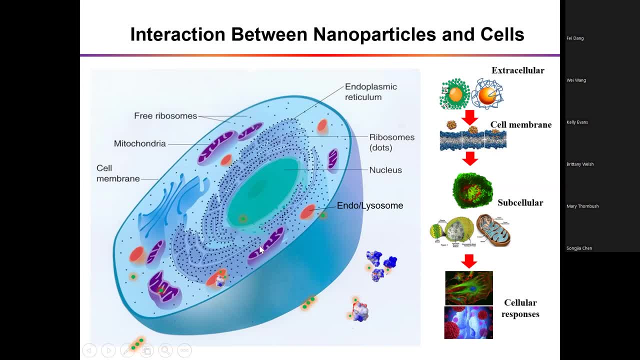 Lianfeng Zhao PhD interface. the third one is the Lianfeng Zhao PhD Is the chemical reactions at the surface of nanomaterials, because other ones, Lianfeng Zhao PhD, know the end of some unless i'm a ecstatic environment and there there are others, other results and them inside the cells. so they suggested that then mature me. 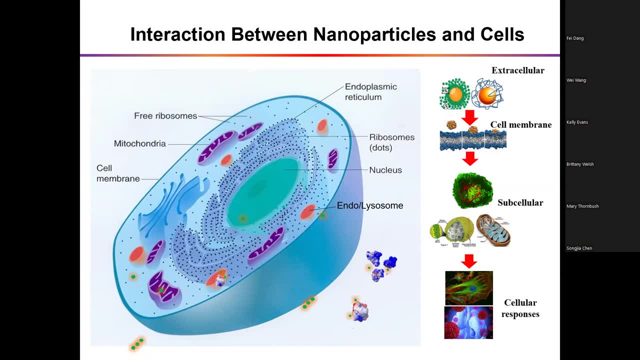 Lianfeng Zhao PhD. involved in some chemical reactions. Lianfeng Zhao PhD. So yeah, so we need to know what happened at the chemical reaction for nanomaterials inside the cells. Lianfeng Zhao PhD. From the whole. 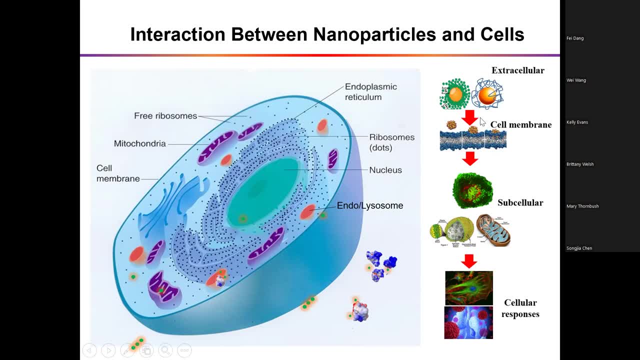 Lianfeng Zhao PhD picture. we need to to answer several questions at a different levels. why protein lipids? another is the inside of sales and Lianfeng Zhao PhD? Because the complex of the integration and we we need a different ways to capture the interactions, one way that we 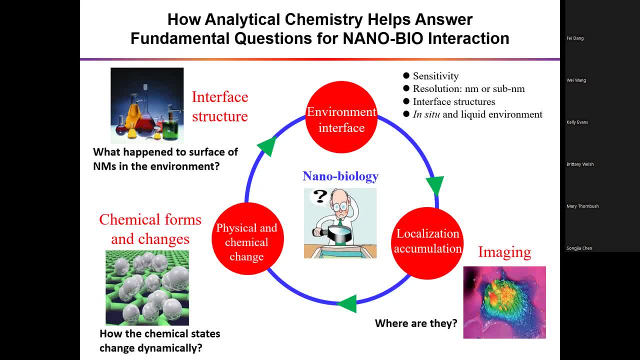 Lianfeng Zhao PhD. First, that we need to know that when that particle go to the specific or micro Lianfeng Zhao PhD. environment. Lianfeng Zhao PhD. What kind of interaction at the interface on that mature- because nanomaterial surface claim major euros when the quarter cost the public, cities and into the some effect the surface, the even. 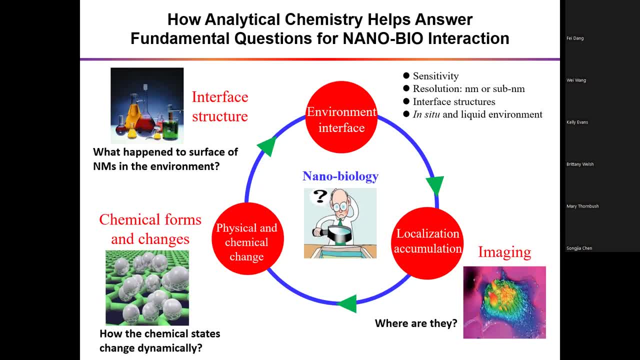 Lianfeng Zhao, PhD. very important. so when you then know what happened to the surface of nanomaterials second night, when the medical inside the sales or in the body we not want to know their distribution. so imagine the important. 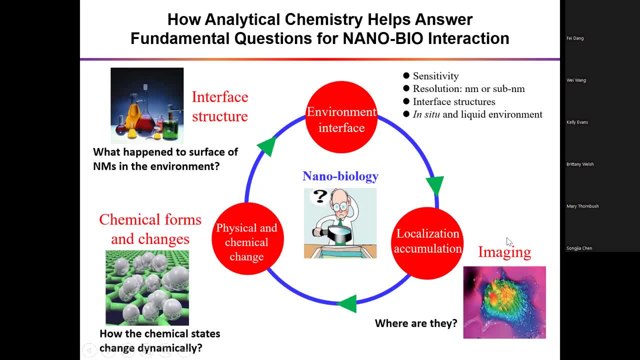 Lianfeng Zhao PhD. important to know the distribution of nanomaterials. third one is Lianfeng Zhao PhD. Then the material is not a inert. sometimes they are chemical and reactive. so we we have to know what kind of chemical reactions to the nanomaterials and what. 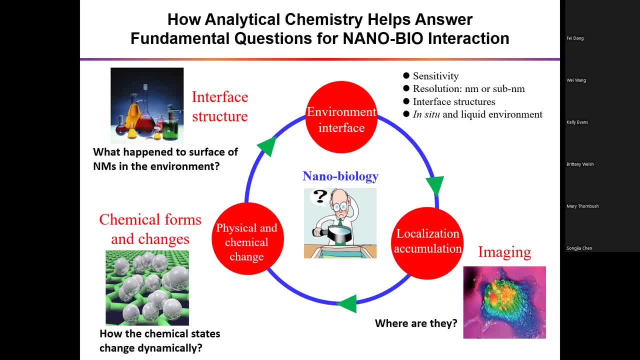 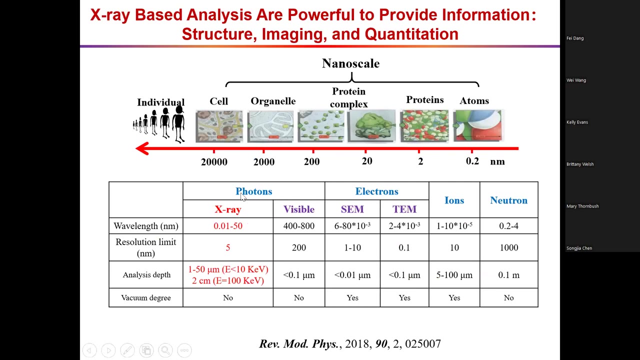 Lianfeng Zhao PhD. What the results of the reactions and the outcome of the ballot? ballot outcome of the reactions. and that means that we need to? Lianfeng Zhao PhD, capture the chemical forms and the changes of nanomaterials inside the the ballot system to answer the fundamental questions. we need to use this on powerful techniques. other window x three based the x three based the techniques either excellent on first to study the elements and 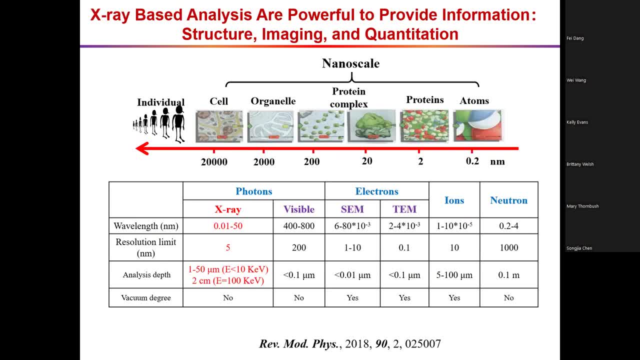 Lianfeng Zhao PhD. elements. they can identify elements in completely complicated system. Lianfeng Zhao PhD. They can also Lianfeng Zhao PhD. They can also detect the electron, electron density to distinguish the monocular, given a monocular at different matters. so the studies that they can distinguish the chemical forms and the chemical valence of elements. so the one that extra x three. however, 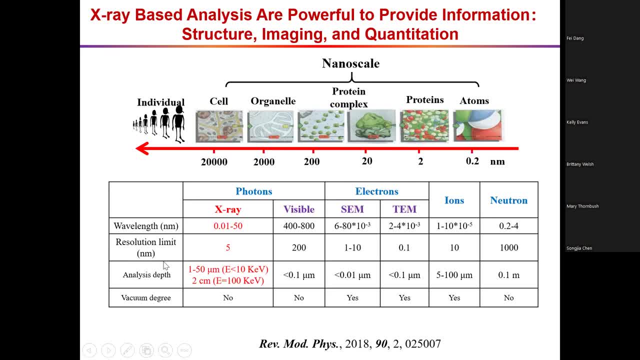 Lianfeng Zhao PhD. Excellent ability to penetrate the samples that we have the the issue of Lianfeng Zhao PhD. They can penetrate our samples with a much higher depth but for visible, for visible visible net and the electrons of the ability, the week the harder need to penetrate or sales. so that means that the x ray can can be used to do 3D. imagine for single sales. 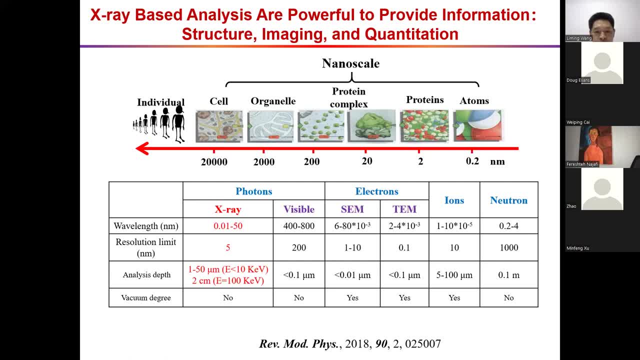 Lianfeng Zhao PhD. So Lianfeng Zhao PhD, So actually Lianfeng Zhao PhD, The powerful. to get a Lianfeng Zhao PhD And not only to obtain imagine information making, also to do structure and a structure for, and then mature and and monoculars. 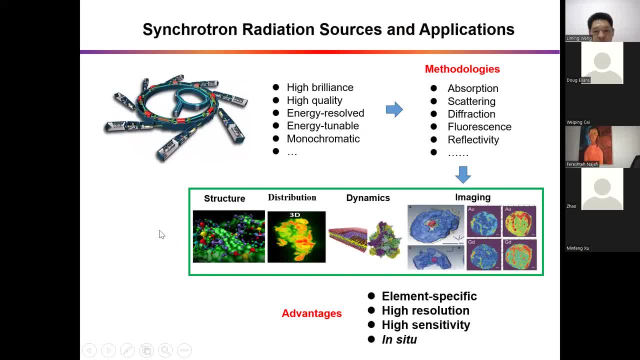 Lianfeng Zhao PhD. So this is to how to get a on how to get the high quality x three on single relation is a facility that can provide a very, very high Lianfeng Zhao PhD, brilliant and high quality x three that the energy x three have, energy reader without the energy to level and monochrome much medical. so this is a very high quality. 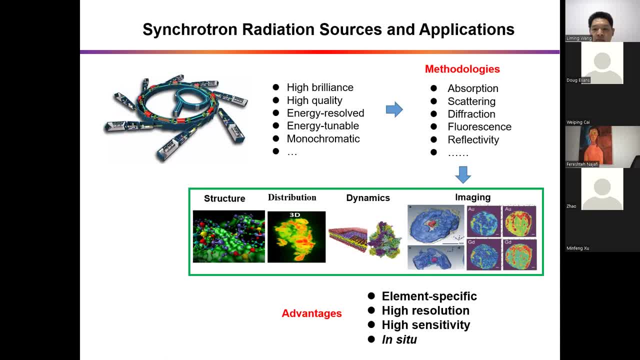 Lianfeng Zhao PhD X three can be combined with some methods, such as the spectroscopy and gathering and imagines. so with this method and the Lianfeng Zhao PhD High quality x three, we can do. 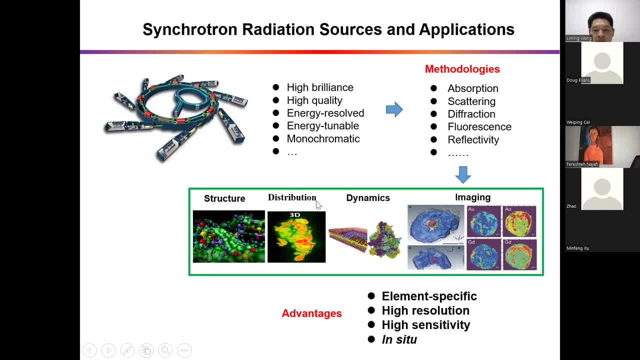 Lianfeng Zhao PhD, Many study for structure and distribution of elements and the dynamic or monoculars, and also for nanometer and then the monocular interactions. you can also to imagine the elements on then, Lianfeng Zhao PhD, Then the materials that you inside the cells, inside the, the single sales and the tissues. 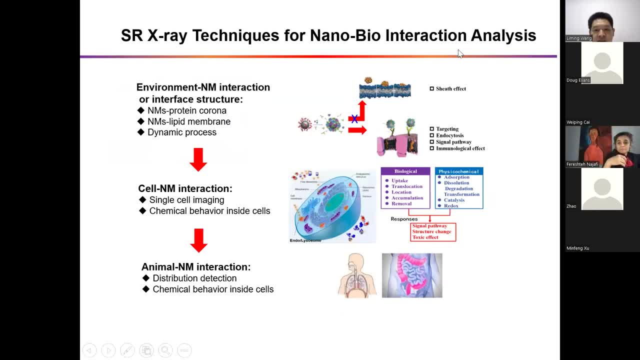 Lianfeng Zhao PhD. So we make a summary about the techniques for nano and by the interface, Lianfeng Zhao PhD- Or here we want to Lianfeng Zhao PhD- highlight to the nano bio interface. we highlight the interaction and interface at the three levels. why is nano? and the micro environment? 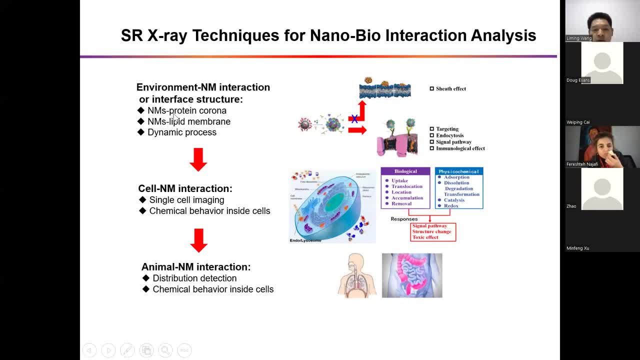 Lianfeng Zhao PhD. interface such as a nanometer with the interaction with the protein and nippets. that is the very directly interface. second is the chemical reactions of nanomaterials. Lianfeng Zhao PhD. Inside the 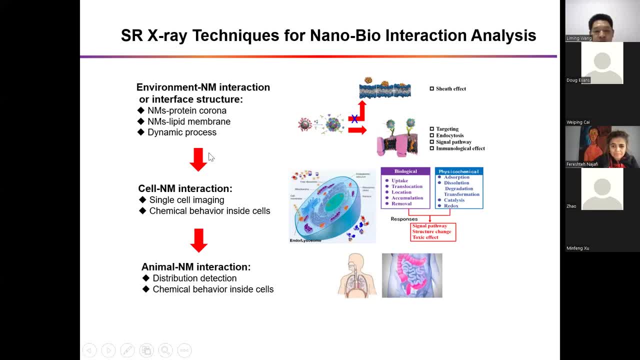 Lianfeng Zhao PhD, cells or inside the tissues. so the second interface that either what happened to the nanometer, other to the surface, or nanomaterials when the Lianfeng Zhao PhD, When the chemical reaction happens, so we capture the. 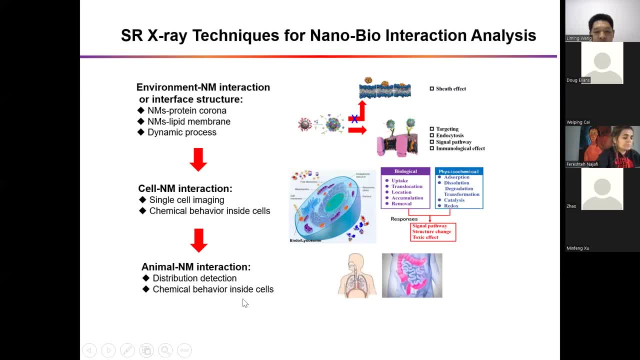 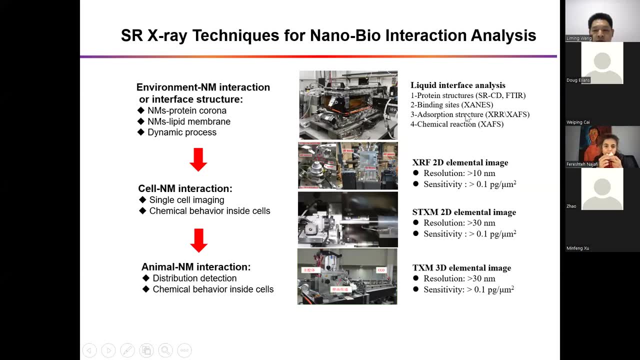 Lianfeng Zhao PhD. chemical reaction at a single cell level and at the animal levels. Lianfeng Zhao PhD. To to know the process that we developed, we developed a server, kind of Lianfeng Zhao PhD. Several methodologies. why, for example, for a nuclear interface? in the message we can use the as. 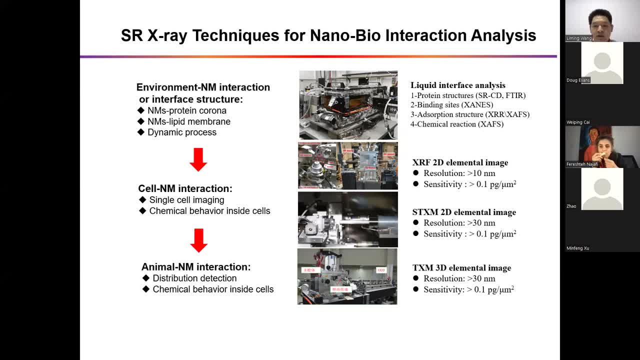 Lianfeng Zhao PhD Synchronization CD and the FTA are to detect a protein structures when before and after in the interview with protein. second, that we can use the x ray absorption of the Lianfeng Zhao PhD spectroscopy to detect the binding site of nanomaterials with the with some protein. 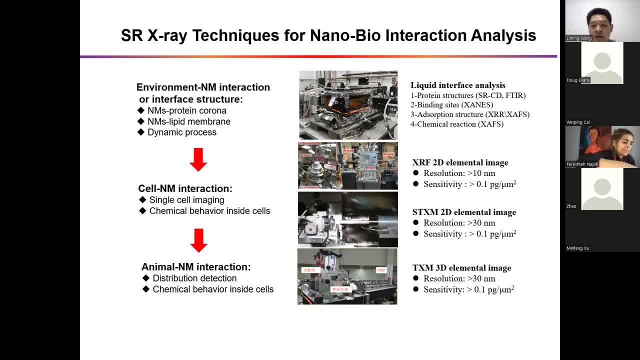 Lianfeng Zhao, PhD. When the protein from the heart corner on the surface. so the one we can use the x three and reflectivity to detect the holiday material interview, interview with the nippy to detect the nippy, the structures after the assumption. so the one we would. and the fourth one we can use the x three absorption. 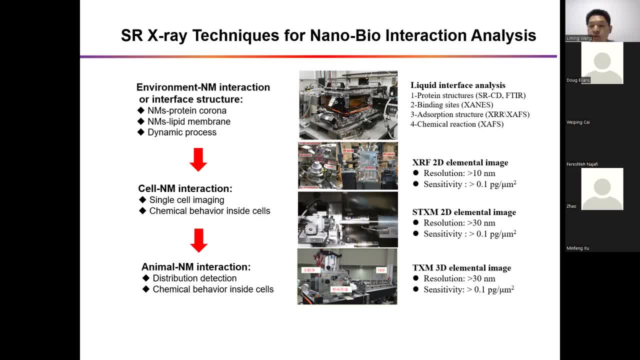 Lianfeng Zhao PhD. x three absorption structure to detect Lianfeng Zhao PhD. To the inner, inner typical interaction for nanomaterials in some Lianfeng Zhao PhD, Some Lianfeng Zhao PhD. chemical, chemical in the environment, for example, and some and some environment, what kind of chemical, what kind of degradation and the chemical states happened to tune in and materials. so they see: the first the nuclear interface and analysis, and other is the for imagine techniques. 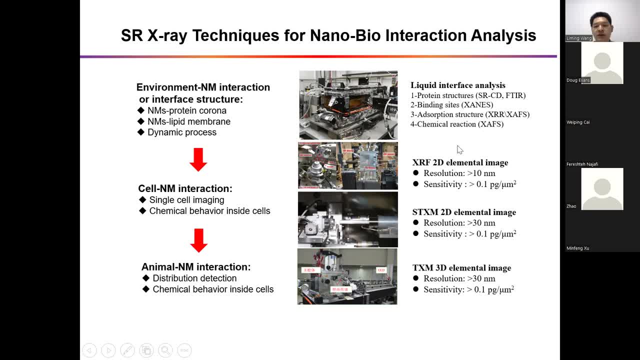 Lianfeng Zhao PhD. You maintain it can detect the in situ chemical reactions of nanomaterials. for example, Lianfeng Zhao PhD, We can use the x, three x three florence little method that can use the 2d scanning for an elementary imagine. they can achieve a high resolution and have a high sensitivity to the day the elements inside the cells or tissues for 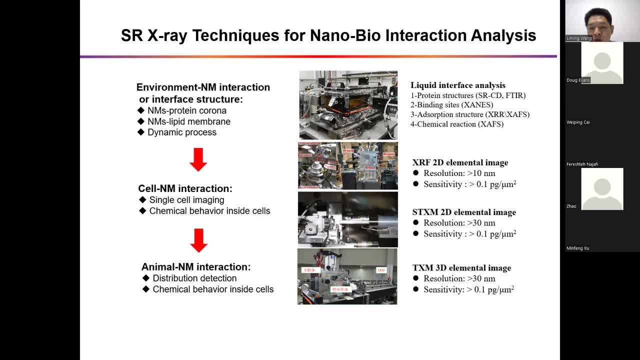 Lianfeng Zhao PhD For another, scanning transition x three macroscopic that also can do 2d or 3d element images and they can have a high resolution and high sensitivity. they can also detect the distribution of Lianfeng Zhao PhD elements, different elements with different the chemical forms. for example, for everyone, everyone, violence to or when three. you didn't make techniques working. 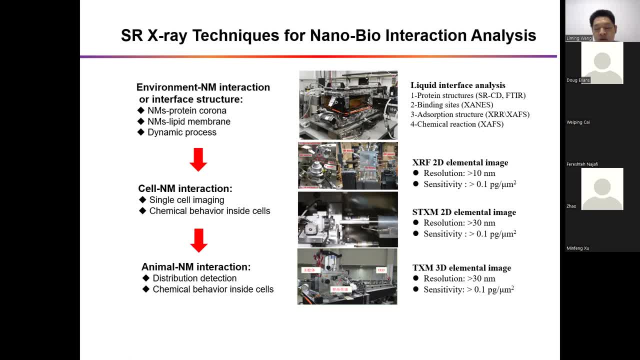 Lianfeng Zhao, PhD. You can see on the the different that you to be able to have a two valence of irons inside ourselves. so this is this powerful for detector, the chemical forms distribution. the third one is the transmission x three macroscopic. the techniques are either very is very powerful to get a 3d imagine for elements because they didn't. 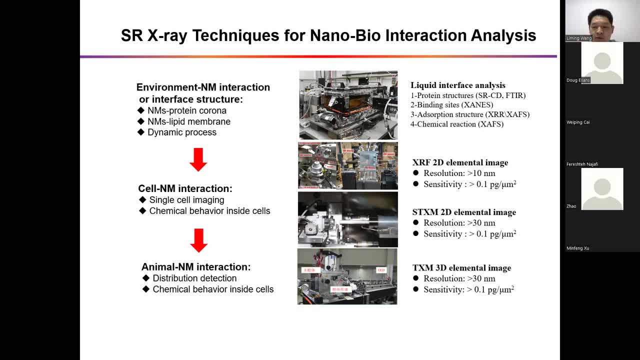 Lianfeng Zhao PhD. Take me to use the x three to Lianfeng Zhao PhD. Try to meet the samples: the Lianfeng Zhao PhD, The. then the sample rotates and for for 180 degrees. 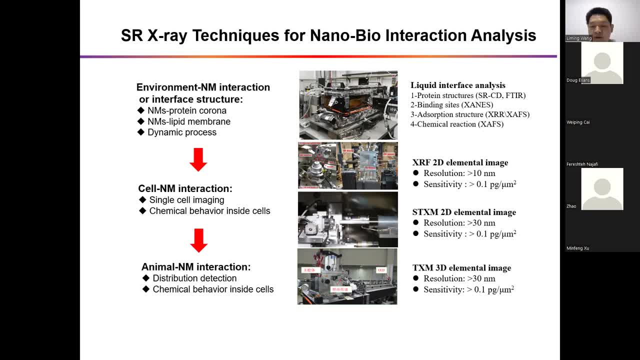 Lianfeng Zhao, PhD, Then we can can reconstruct the figures to get us ready. imagine for for the samples, the why use them? we are using the method to detect the distribution of nanomaterials that are single sales or single. 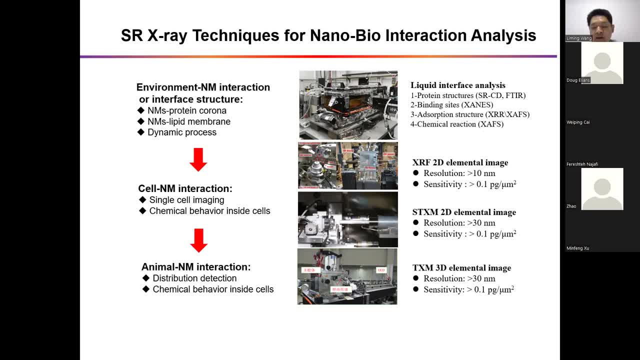 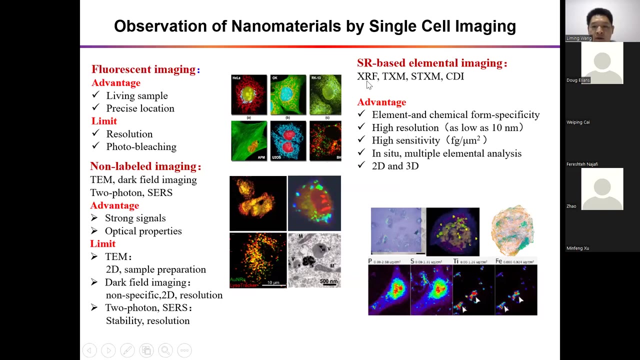 Lianfeng Zhao, PhD, A single on heather particles. so basically this is imagine techniques and a liquid interface analysis. we've study different nano bio interface and structure and the informations and the. this is our Lianfeng Zhao PhD High resolution x three imagine techniques. 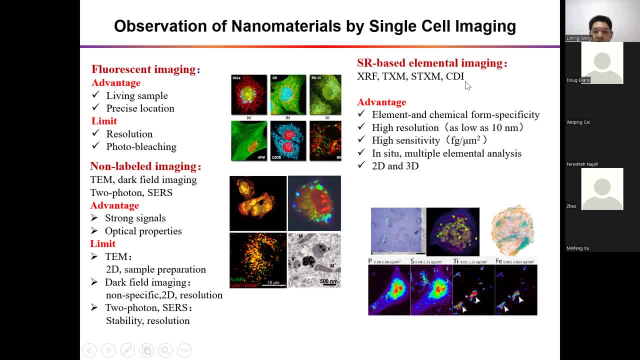 Lianfeng Zhao PhD. X, three, xr, tx, m and stick some and cdi. this method: I have some of the quantity and then have more. Lianfeng Zhao PhD. Abundant is in the Florence imagine and the non labeling imagine, for example, the city for elements, elements specifically imagine- can be obtained that by move over them, but for the no need to enable the particles. 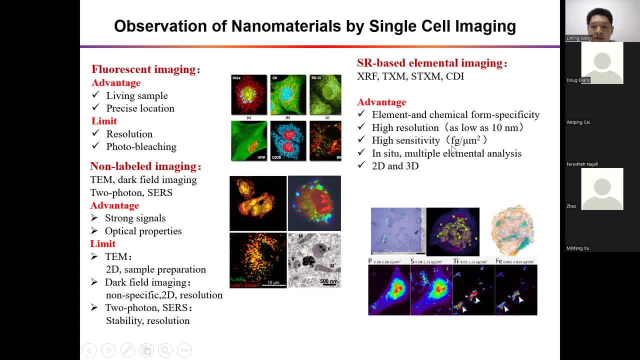 Lianfeng Zhao PhD And also the high sensitivity to rigid is the high Lianfeng Zhao PhD female gram per per micro meter square. so they can also to study the in situ chemical reactions for the sales. 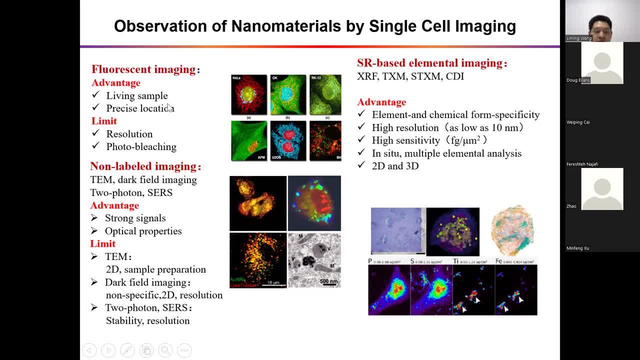 Lianfeng Zhao PhD. But for the Florence imagine. the also have some of the value on. even sell on him sample imagine. but the limited is that the low resolution and the will be a need. some labels Lianfeng Zhao PhD. They cannot to detect the chemical reaction or nanomaterials that sales. 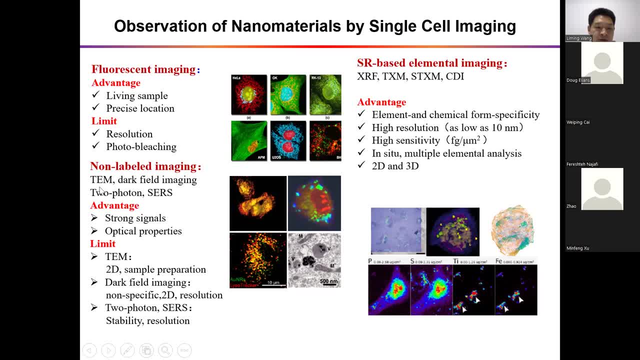 Lianfeng Zhao PhD For other non labeled and imagine, for example, tm and other techniques, and they needed to. Lianfeng Zhao PhD, The the how they need to penetrate the samples and they cannot get a. 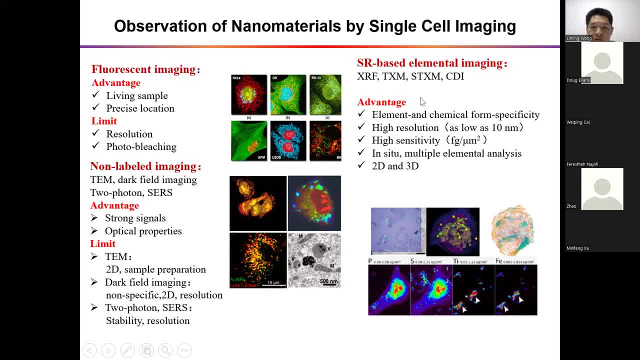 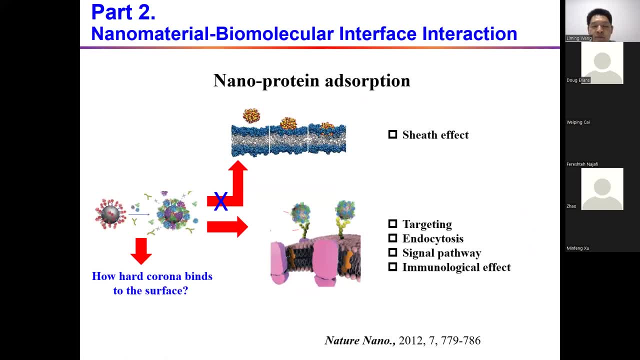 Lianfeng Zhao PhD, Get the in situ information. so with the other one to do, we were introduced to tears on examples of for how then the techniques be used in nano bio interface? Lianfeng Zhao PhD studies, and the first example is that about nano protein absorption and interaction. but the window when that particle in 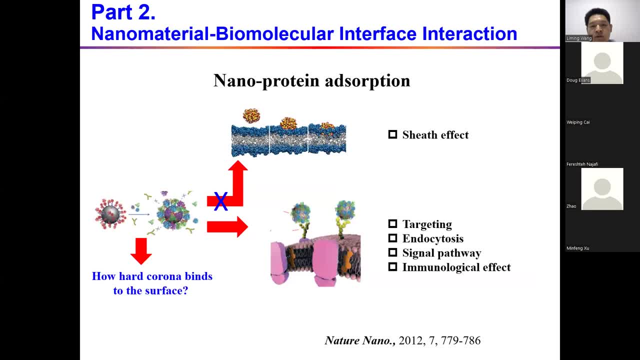 Lianfeng Zhao, PhD, A before that particle integrated with sales. they were first taking her with all the protein and around the sales: the protein. some protein have a form of something on surface, some are have a loose. Lianfeng Zhao PhD Assault on surface. love from the assault. the protein called the half corner. 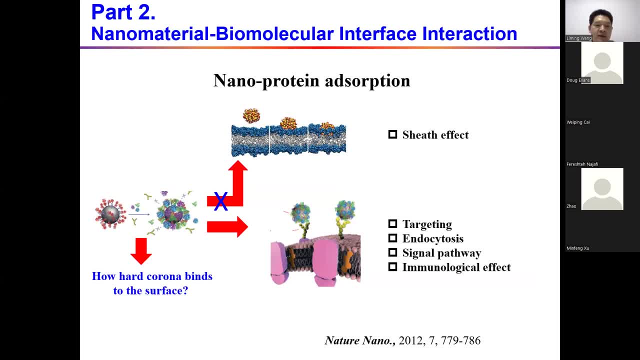 Lianfeng Zhao PhD And other one know the heart corner play a very important role to prevent the toxic of the toxic surface on the materials. but the structure- Lianfeng Zhao PhD structure is not clear. 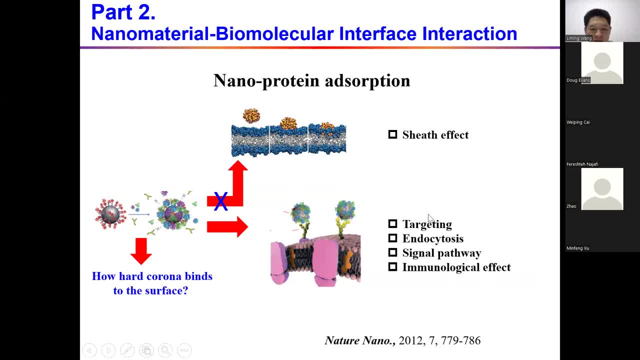 Lianfeng Zhao PhD. So when we- yeah, if we can reveal the bedding structure for nano and protein directly, we can best, the better us than the horn and the material. how, putting corner quarter some value factor, Lianfeng Zhao PhD- And the trigger some, some effect, neck inflammation, like a signal pathway on activity activations? so to answer the question, we, we 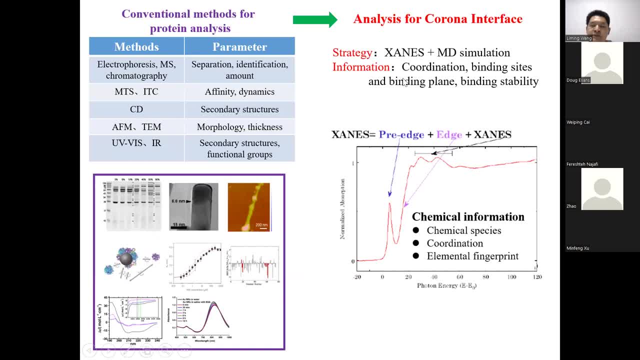 Lianfeng Zhao PhD. Do not develop a new message with based on x three on x three on near edge, so very close to copy. the techniques on can be combined with the Lianfeng Zhao PhD. molecular dynamic. 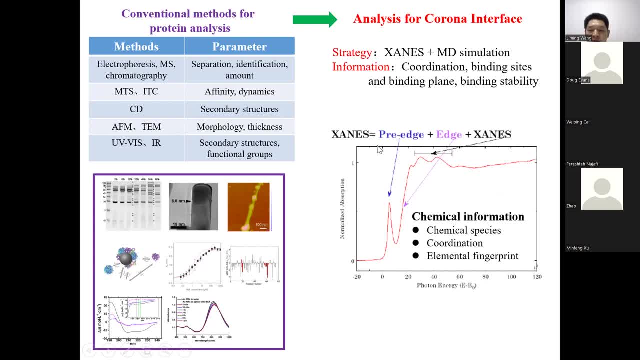 Lianfeng Zhao, PhD. We can leave the message there can be detected as a chemical information of the elements. they can detect that the chemical specialization, co, chemical coordination of the elements. they can also serve all the elements of fingers print to be based on this. 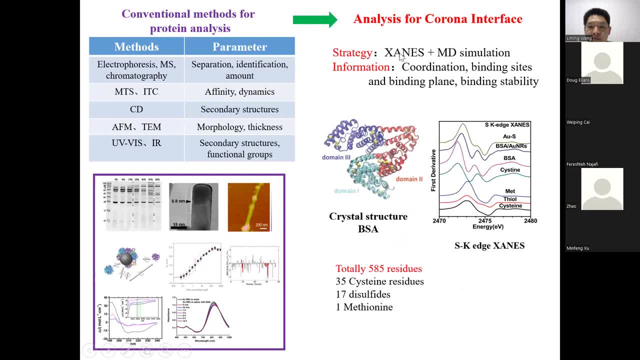 Lianfeng Zhao PhD Advantage. we can use that this method to detect a different chemical forms of software inside of the albumin. the albumin have different Lianfeng Zhao PhD properties. Lianfeng Zhao PhD So. 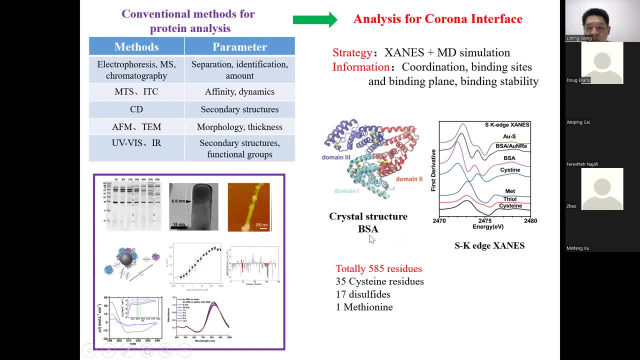 Lianfeng Zhao PhD, The kind of before and after interaction. the albumin, Lianfeng Zhao PhD, The software chemical form change for them. at the beginning we have a user site or software. then after the interaction that it's our fad that were break and in and into the matter. if the interview to the matter element and that particle there were from the mentor software bond and Lianfeng Zhao PhD. Different Lianfeng Zhao PhD. The kind of Lianfeng Zhao PhD Before and after interaction, the albumin. Lianfeng Zhao PhD, And then we'll suffer. have different the. 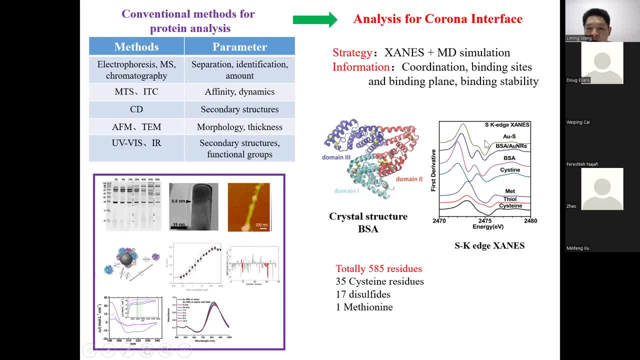 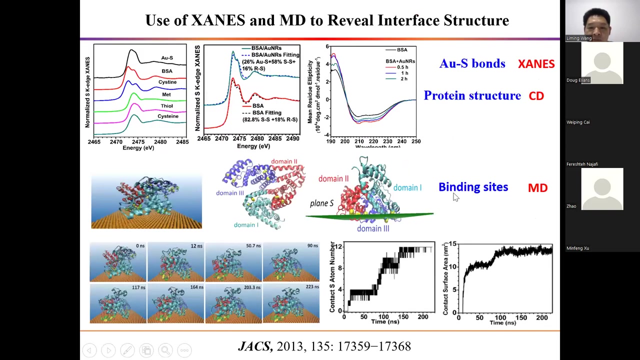 Lianfeng Zhao PhD and Lianfeng Zhao PhD Given the spectra fingerprint, so based on the fingerprint that we can calculate what the ratio before and after of the Lianfeng Zhao PhD protein in the room that was the goal of the particle they. they can be used to quantify the software chemical forms based on the colony vacation information of of that. 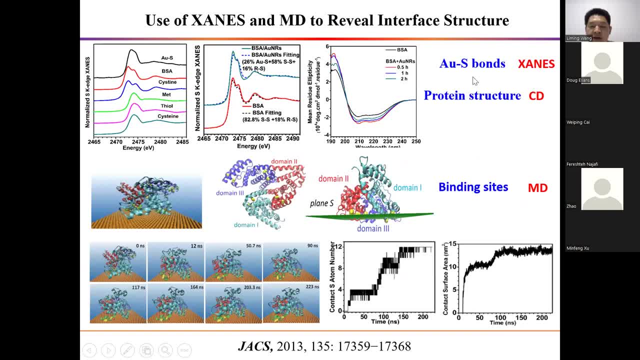 Lianfeng Zhao PhD. We can, Lianfeng Zhao PhD, Detect how many and you suffer that break. then we can use the MD simulation. the simulation can detail the work with the actual and that location. Lianfeng Zhao PhD. Actual. a new location of the protein in her writer. with the net particle, based on the two bits, on the two ways, we can detect how the in the register as the surface of the gold. so 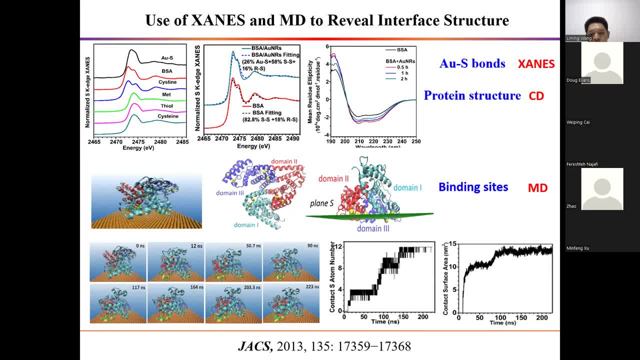 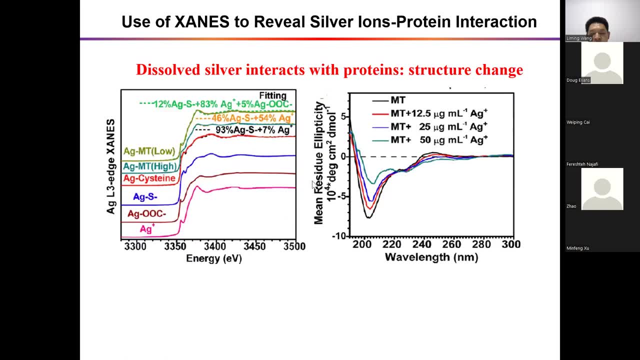 Lianfeng Zhao PhD. That is a very good way to call it. qualify protein and nano integrated at the interface? Lianfeng Zhao PhD. It says that the answer. we can also study other men and the material, such as a seven and a particle. seven and a particle can also with some proteins. the empty is. the is is a protein that can interact with the matter and being quenched, the 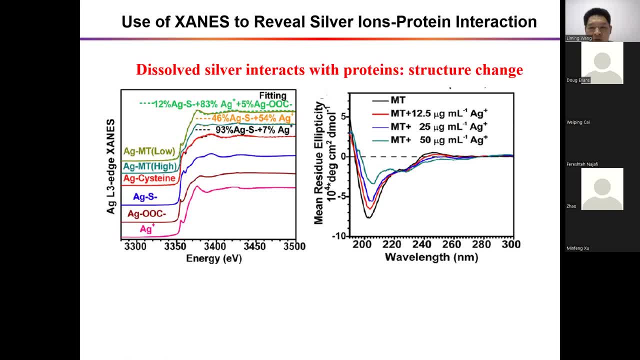 Lianfeng Zhao PhD. The Lianfeng Zhao PhD On Lianfeng Zhao PhD And do, but by value of the 16 group sitting sitting on mine assets. so you, this similar method that we use the srcd and the jobs we can detect and what how, the protein in changing the structures and and the shoe, the bed inside, over the proteins. 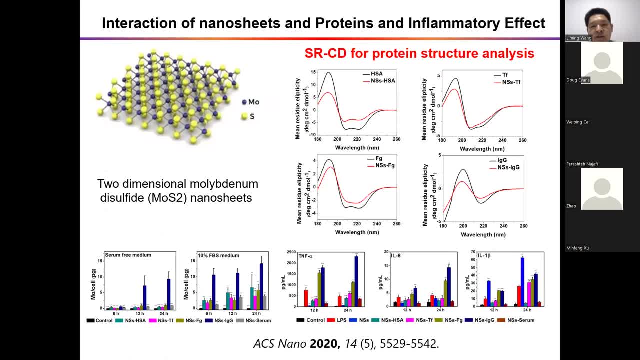 Lianfeng Zhao PhD. More Lianfeng Zhao PhD. We can. we can also use the srcd CD to to to get the protein thickness structures. Lianfeng Zhao PhD, Are the the thickness structure either? 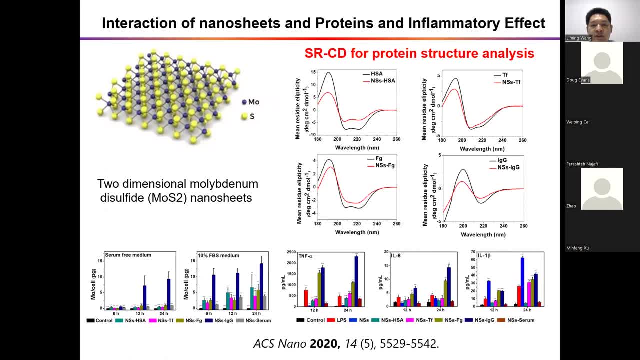 Lianfeng Zhao PhD At our city. the more powerful than traditional CD because the CD can get a much lower on wavelength than the traditional and city to the city can only from the Lianfeng Zhao PhD 190.. 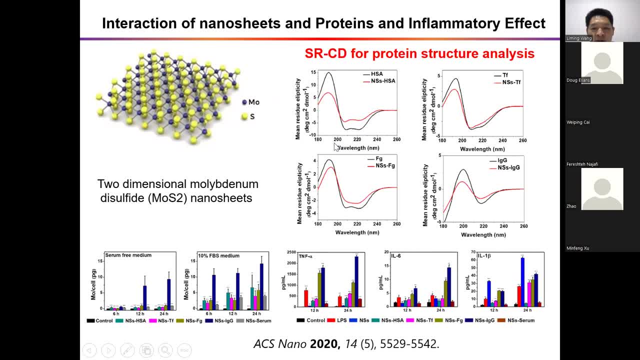 Lianfeng Zhao, PhD. And then these srcd can reach the 160 nanometer, so on between 160 and 190. there are many details, signal structures, and so based on the details, structure we can calculate and the feet, the structure that between after and before and after in the record proteins, they can get them more detail structure information. 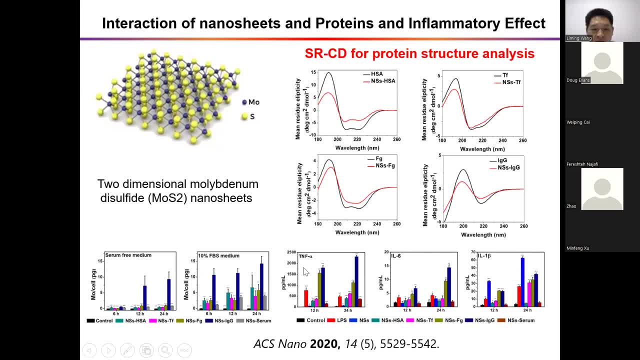 Lianfeng Zhao PhD, And more Lianfeng Zhao PhD, Over for srcd. we can also detect their interaction with the proteins and so, based on the srcd, we study on the one, two dimension money. 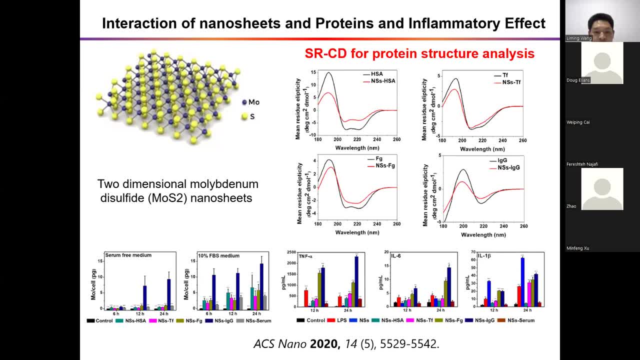 Lianfeng Zhao PhD, More money and the norm on the surface and then state in the roses kind of for kind of proteins. working on of the of, we can observe, Lianfeng Zhao PhD, That the protein 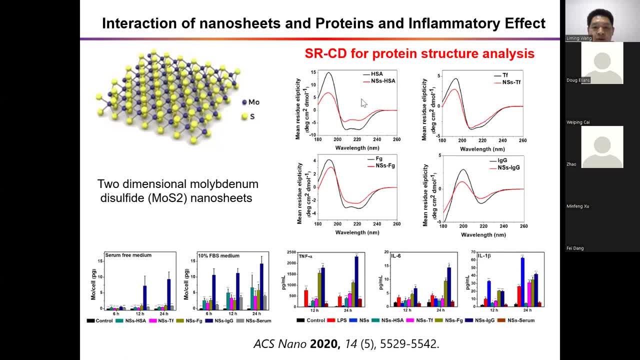 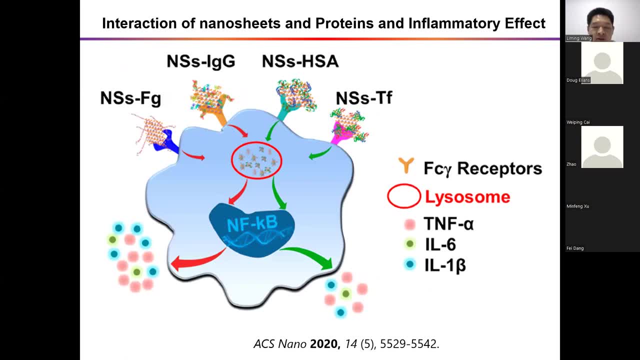 Lianfeng Zhao PhD To need a second structure after the assault on surface. Lianfeng Zhao PhD, And based on this structure we can conclude the hall and mature trigger the inflammation. so the structure is very important to shoot the making them. 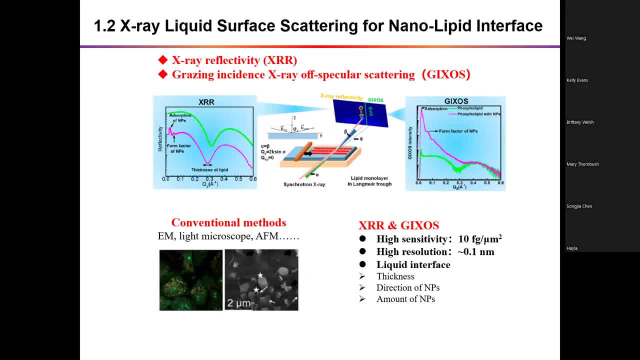 Lianfeng Zhao PhD. Next, though, we we use the liquid, the surface of the gathering, to study how many material in terms of the nippets, and we, Lianfeng Zhao PhD, This X three reflect activity and the defaults are to kind of powerful scattering method to study what happened to nanomaterials and the nippets added on the surface of in a separate liquids, the tune that this tune techniques can be used. 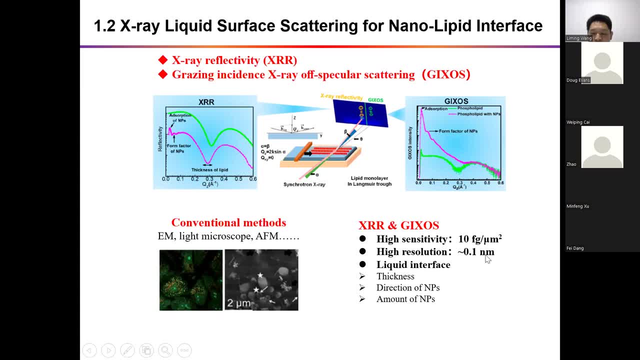 Lianfeng Zhao PhD, To provide a high finitive and high resolution informations. then the Commission, Lianfeng Zhao PhD. Our method, for example. we, for we started in the nature of the internet, between the nature and nippet that we use the. 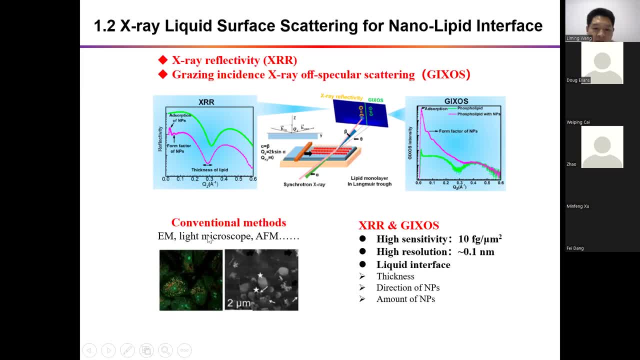 Lianfeng Zhao, PhD. Electron, you natural math to copy and another micro, so copy. and the FM are the semester that some, most of the time the even try. the environment also the imagine neither. some dice to stay, the sustain the samples. they are not the real information. so 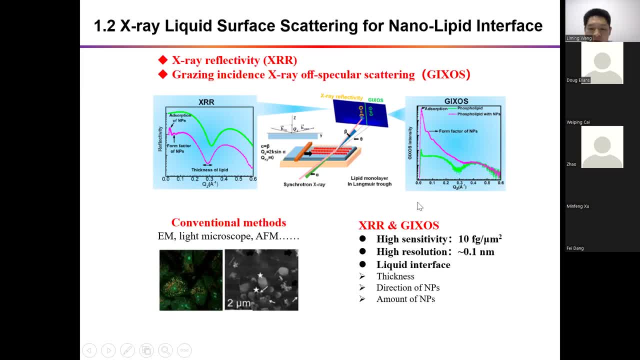 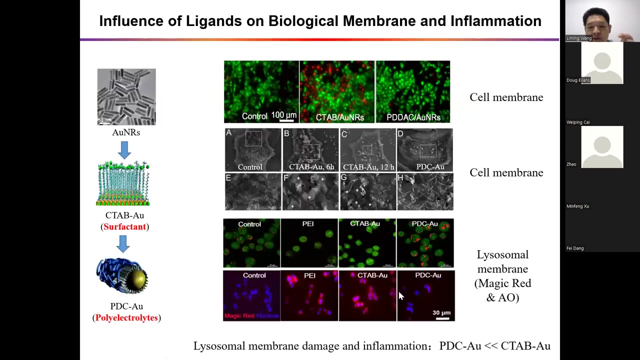 Lianfeng Zhao PhD. We based on the liquid techniques that can provide the Institute of nuclear Lianfeng Zhao PhD Environmental structures, so that structure, including the sickness of the nippets and the directions of also the net particle and then the amount of the nanoparticle on the surface of any nippets, based on the information we can study, calling the material structure or surface. 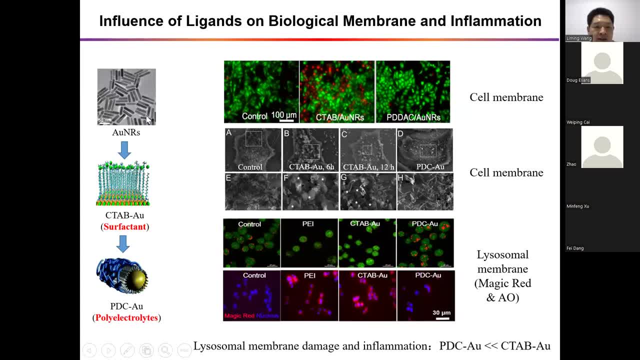 Lianfeng Zhao PhD. affected. Lianfeng Zhao PhD. The nippy, the structures. for example, we started a goal, not the roads and this goal either have different the curtains. Lianfeng Zhao PhD. Why is the certificate in the equity that they see tap go that road? we have a barrier structure on the surface of go the father, the value of the, you know, stable. 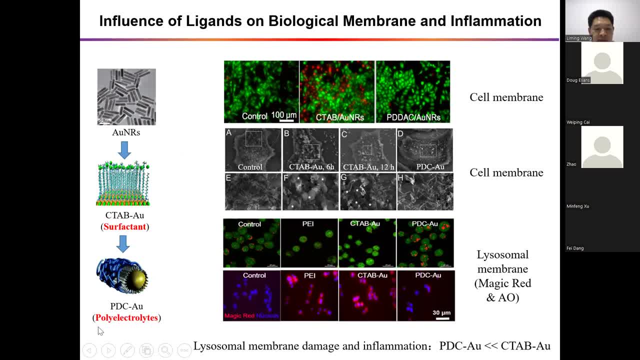 Lianfeng Zhao PhD is not stable. another model modification is the pony like electrolytes lead. the modification is based on the on the tape and another Lianfeng Zhao PhD Negative surface, so by near by layer on a seven. in this, the important in X right maybe go to the surface of the net rod. so to compare: 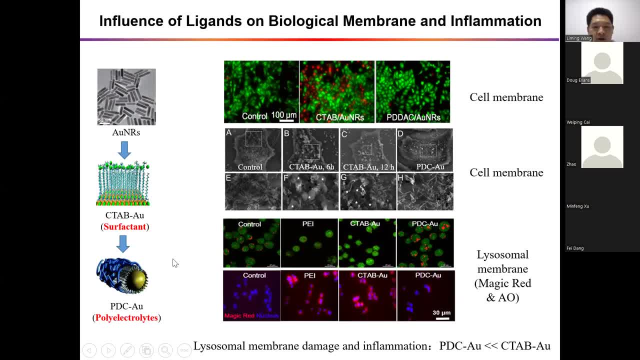 Lianfeng Zhao, PhD. These two kind of coating and the effect of on the sales. we found that the the certificate and the goal and, rather than me, cause the cell death and then the cell membrane on the pony. you like this for nights going on the road, they are safe. 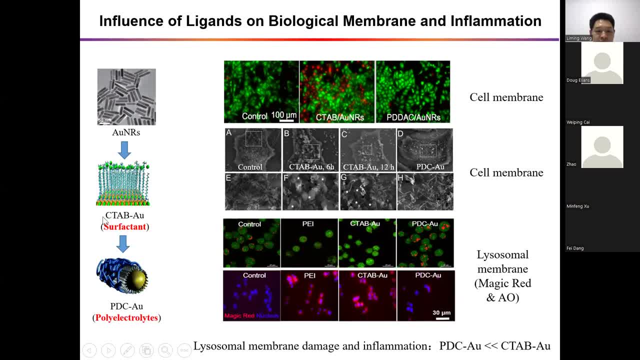 Lianfeng Zhao, PhD, To sales I did in the course. they are death of personal or though they are both of positive charges and monocular, for the way they have different effect on memory. to answer the questions we use the X Ray based. 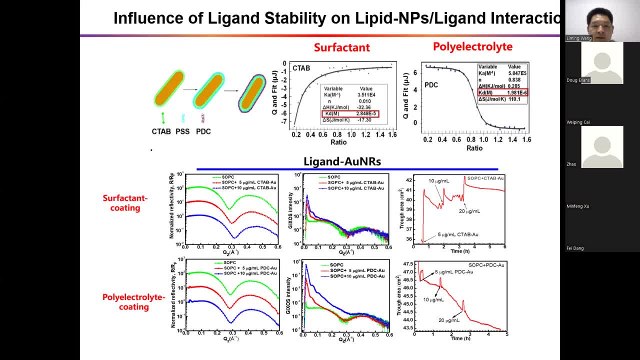 Lianfeng Zhao PhD techniques to study how their interaction happened at the liquid Lianfeng Zhao PhD surface. we use these Lianfeng Zhao PhD See tap go network and Lianfeng Zhao PhD The goal of the road to study their. 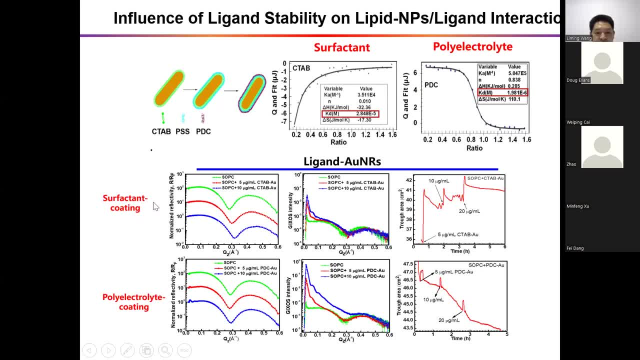 Lianfeng Zhao, PhD, interactions. we found that certificate tender coating and that road may change the thickness of the nippy that. we found that other interaction: the thickness of the nippy that changes. and then we can also get the Connie petty. 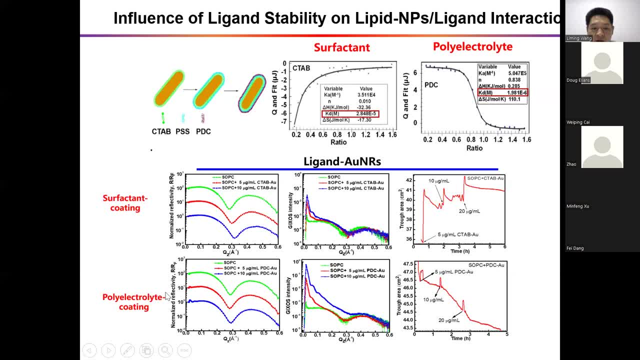 Lianfeng Zhao PhD. Information about the sickness of nippy. Lianfeng Zhao PhD. For pulling you like. so perhaps leave the remain the Lianfeng Zhao PhD. The same thickness of nippy. so such is that these two kinds of monocular modify the goal. that will cause a different effect to the nippy. it. 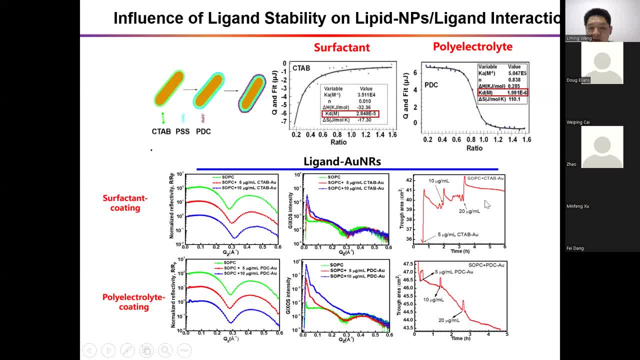 Lianfeng Zhao, PhD. Then we can see that the for the circuit and the circuit and the Cody, then and particle, the, the nippy. the area, trap area in cross increased due to the detect of the molecule monoculars. they were inserted the nippy. 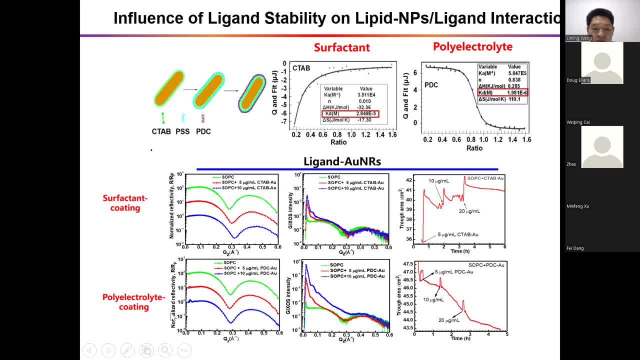 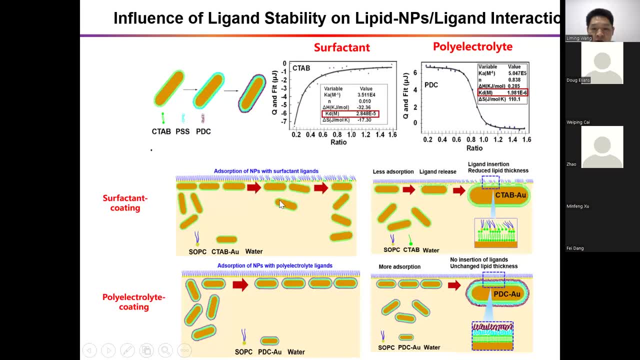 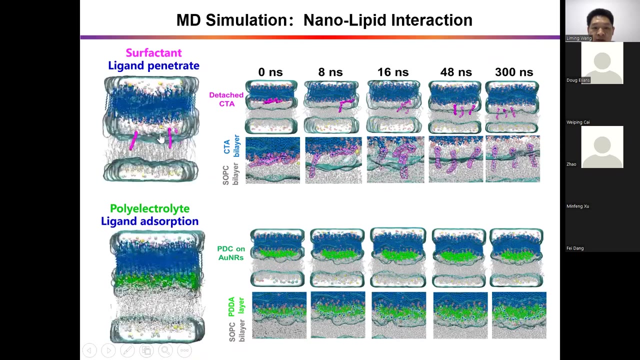 Lianfeng Zhao PhD. But for the one, the didn't change your lot for the area. or repeat: Lianfeng Zhao PhD. We can see the mix them for the two monoculars that they were. nippy the under, inserted the structures and by the stable on the surface. then we use the simulation to study the two kind of Nana roads for safety attention so we can see the negans may penetrate the liquids. 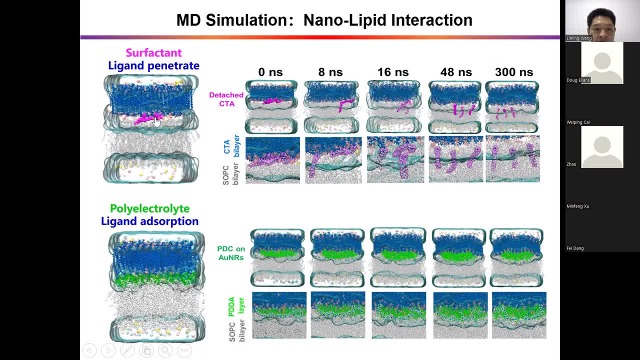 Lianfeng Zhao PhD. A. Lianfeng Zhao PhD. The nippy, the nippy nippy that they use on the city tap monoculars. they can penetrate the nippy and they're changing the structures. and this is the point in actualize the leg and the remainder as 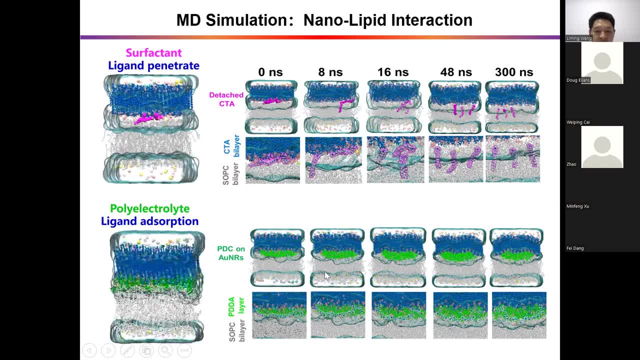 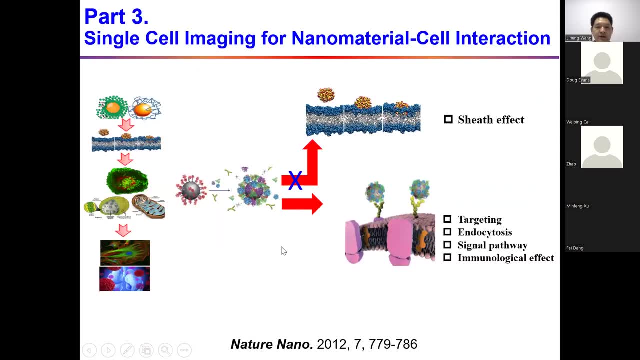 Lianfeng Zhao PhD. Then particle and the nippy the interface, so they didn't change the structure. nippy, the on the course in the next set of the facilities. Lianfeng Zhao PhD. Next, though, I will introduce the application of single sale. imagine for: 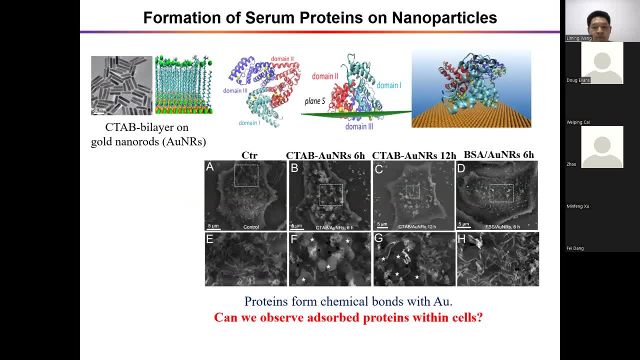 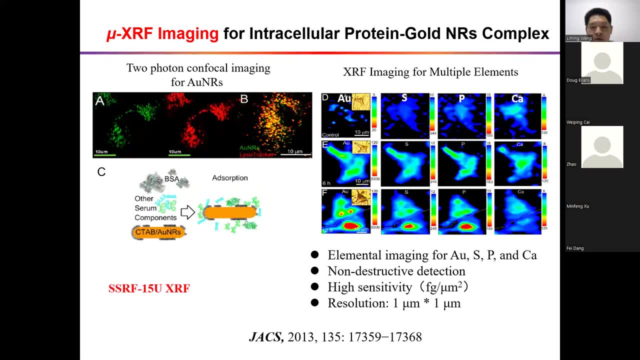 Lianfeng Zhao PhD material and steering directions. Lianfeng Zhao PhD And other window Jeff and now on Lianfeng Zhao PhD. And then mature kink are quoted by proteins before they enter the sales. so we have a question whether we can detect that the protein. 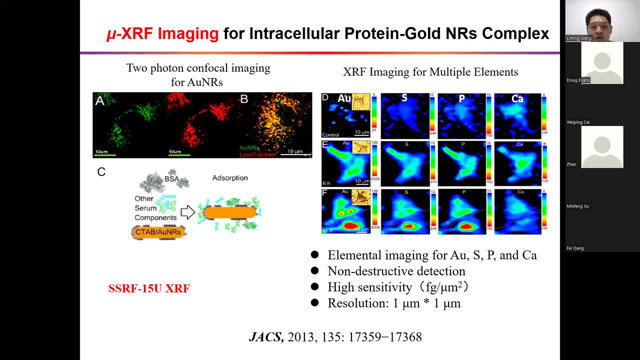 Lianfeng Zhao PhD The, also the protein when they go in the sales. other window: protein continuous. some surface. we use the system. other example: we use a goal, not about the cookie: the Lianfeng Zhao PhD proteins. 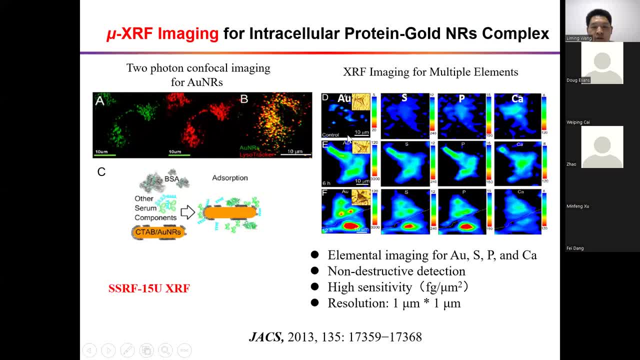 Lianfeng Zhao, PhD, Putting cutie the color to study that interact with the sales. we found that after interaction with sales, the element imagine for good and suffer increased with time. so this based on x three, Lianfeng Zhao PhD, Florence imagine can show that director evidence for nano and the protein corner going to have the sales together. 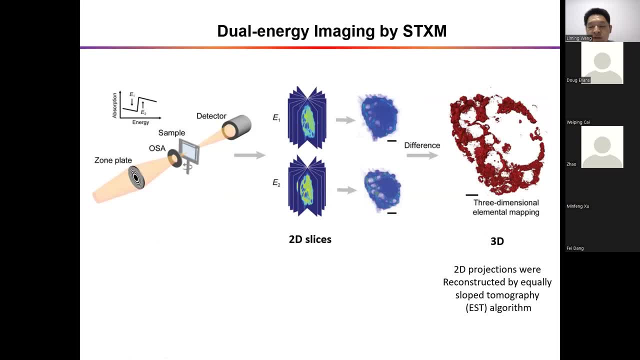 Lianfeng Zhao PhD. And, moreover, and we can use the stick song to sell Lianfeng Zhao PhD- The whole resolution for the particles is especially for some particle had any capture. capture that by tm, for example, and we use this, the kind of chemical. 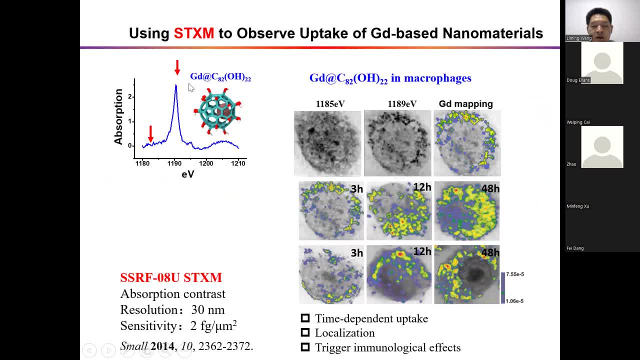 Lianfeng Zhao PhD. This kind of nanoparticle, this particle only contain the one element. what metal elements is how? they need to detect them by tm because of the contrast. Lianfeng Zhao PhD. In the very low. 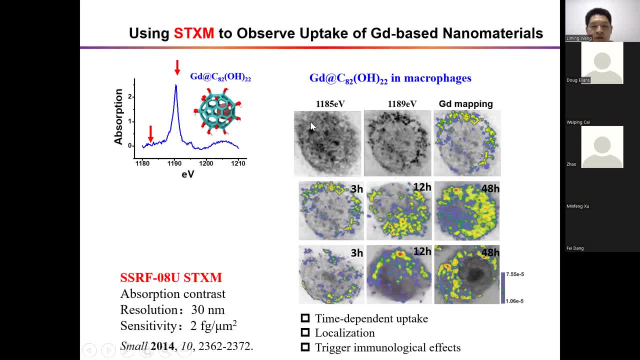 Lianfeng Zhao PhD. 40 m. Lianfeng Zhao PhD. So we think out of whether we we can use the element of based imagine to take a little nanoparticle when the uptick of back with the uptick and by macro, macro feeds, we found that 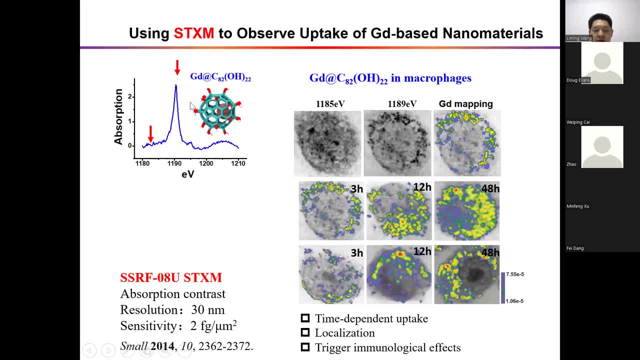 Lianfeng Zhao PhD, This investor that can detect that Lianfeng Zhao PhD can be used to imagine elements and based on the pre age and on the age- and it meant Lianfeng Zhao PhD. absorption x three absorption efficiency. 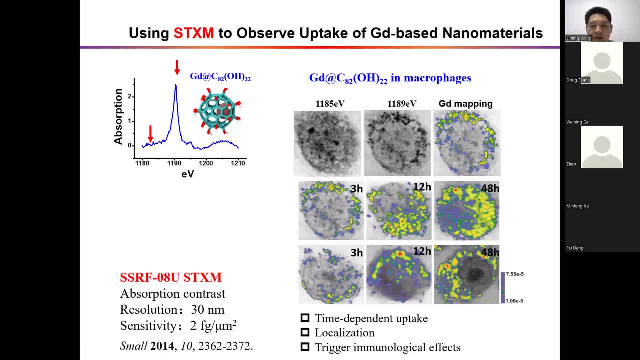 Lianfeng Zhao, PhD, To be based on these properties. we can detect the different energy and the image at a different energy based on the pre age and on the age. we can see the different signals for the samples. then we sub subtract to the signal that we get to the 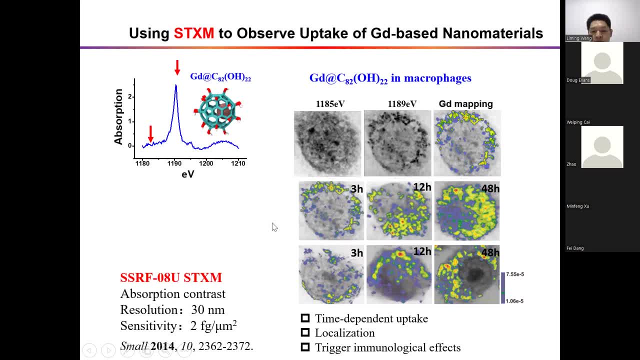 Lianfeng Zhao PhD. distribution of elements. so we use in this investor those study different time. Lianfeng Zhao PhD. At different time, the distribution of elements. Lianfeng Zhao PhD. Inside the sales. so this is a method that can successfully detect the some and some challenging nanomaterials inside the sales. 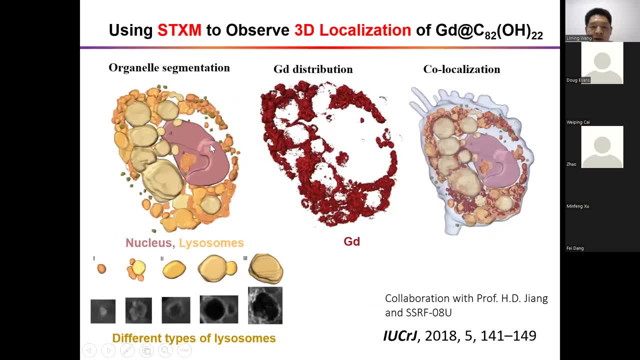 Lianfeng Zhao PhD, And, moreover, we can use the method to do 3D, imagine, to, based on XR, on the stick song, to see the elements inside of the specific organ in nails. and because, Lianfeng Zhao PhD, We use a system and the CD, I working 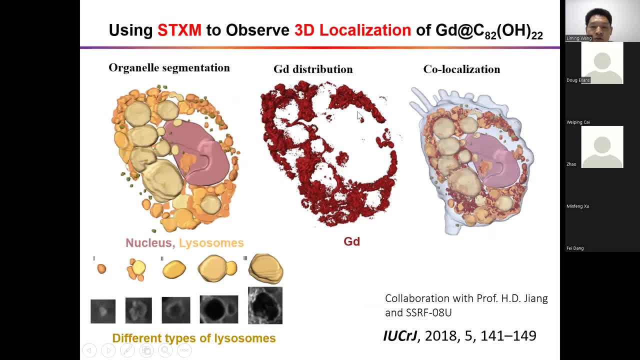 Lianfeng Zhao PhD, The electron density of the samples. Lianfeng Zhao PhD and different. the other land of the South South, such as the new cleaners, Lianfeng Zhao PhD And the some less or much endure. the different have a different. 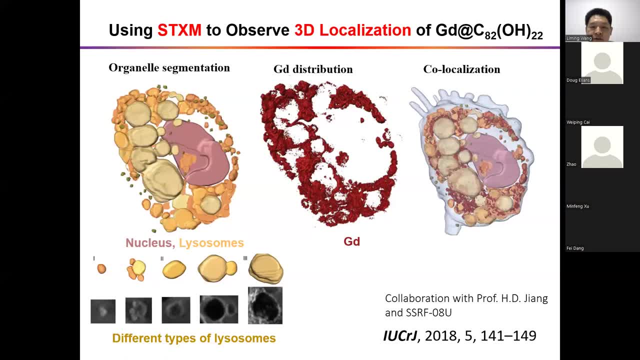 Lianfeng Zhao PhD, An electron in in a 20 core entities so we can distinguish a different or nanos Lianfeng Zhao PhD. Then we pick the X three. if X rf, imagine, we can show the distribution elements. 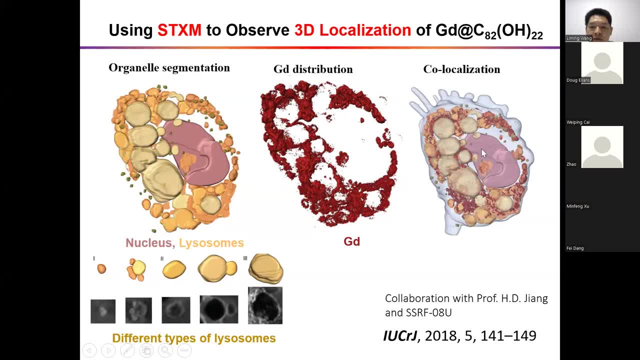 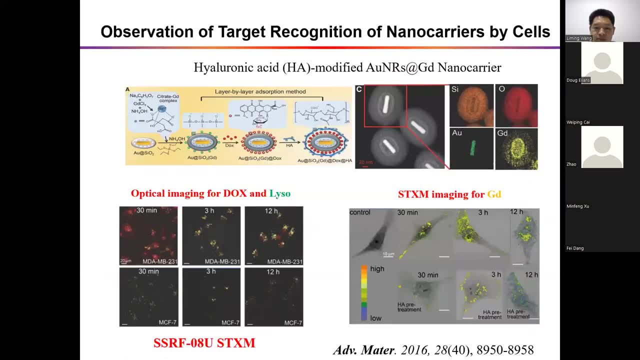 Lianfeng Zhao PhD. Combined together, we can know: Lianfeng Zhao PhD, The collocation of elements as a 3D, imagine as a 3D and level to see the distribution. Lianfeng Zhao PhD, Moreover, with study on other than the material inside the cells. but we can use the investor, that on stick song, to study some matter containing, and then the carrier to study how the target of the tumor sales. 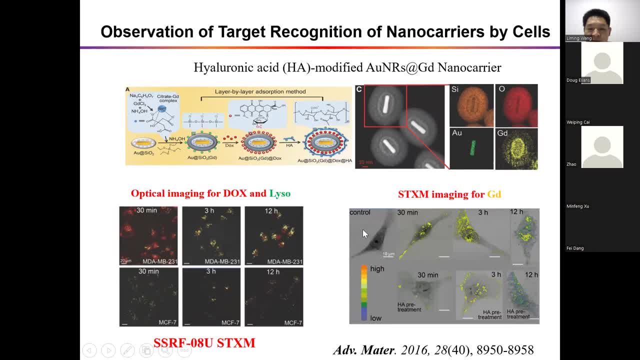 Lianfeng Zhao PhD. Based on getting in the arm elements, we can see the Lianfeng Zhao PhD tumor cell up up, take up, taken the particle with time. if we use the some inhibitor for the receptors, we can find out that the uptick in either inhibited, so suggest that the uptick either. 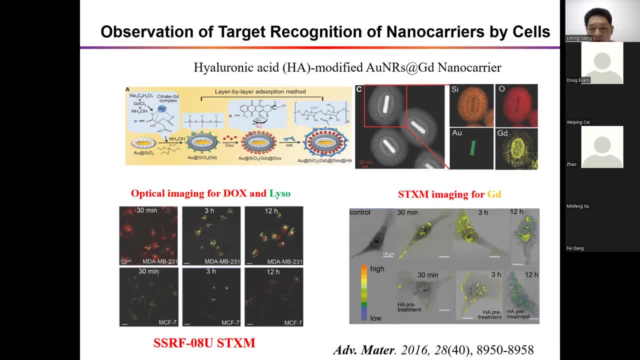 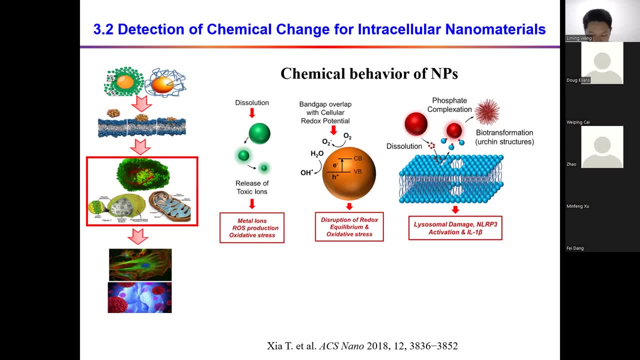 Lianfeng Zhao PhD. Of the net particle, you either bio some receptors. Lianfeng Zhao PhD. Moreover, we we also use the Lianfeng Zhao PhD hybrid. Lianfeng Zhao PhD Imagine to detect the what happened inside the cell. other window: when the particle going inside the inside the cells, the different that. 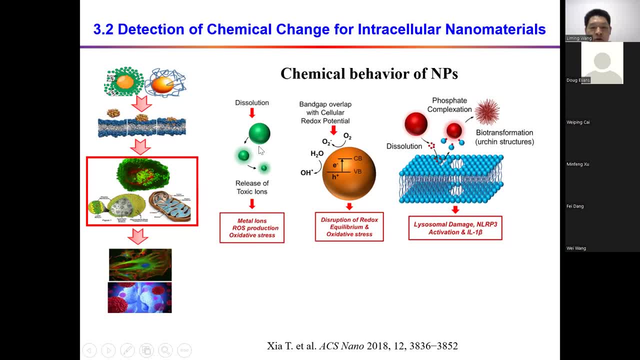 Lianfeng Zhao PhD. There are several different. that can chemical reaction and, for example, somebody talks of the particles. there are some chemical coordination of the Lianfeng Zhao PhD. Some molecules inside the site of the nippets, another maybe they are. maybe also that the into some of the 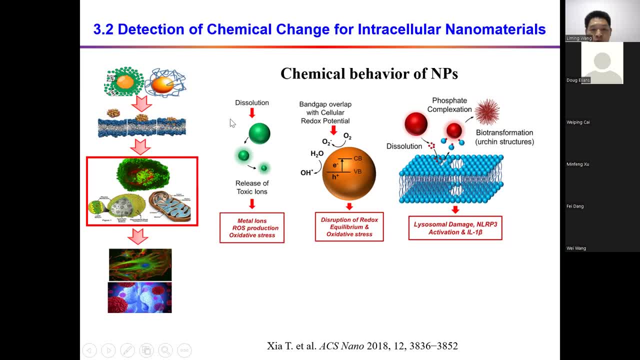 Lianfeng Zhao PhD Audition forms and then they may be resolved in a physical environment to earns. so to understand that what happened to the materials inside the cells, we can use the x three absorption Lianfeng Zhao PhD Spectroscope copy and the x three imagine to detect that the reactions in vivo. 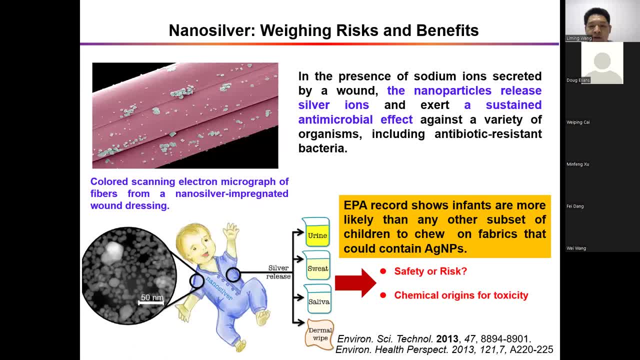 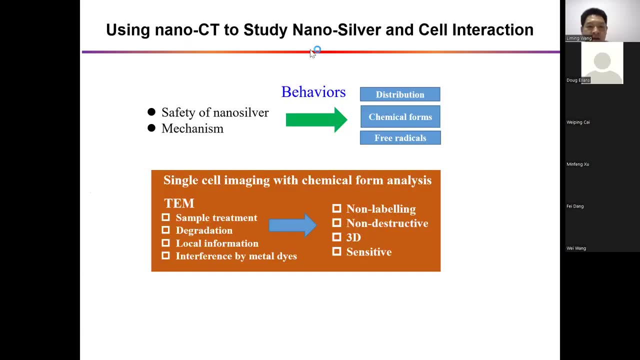 Lianfeng Zhao PhD. Other windows seven. that particle you are considered considered to be toxic to Lianfeng Zhao PhD, To sales and to home beings. however, the chemical reaction making them even steer know the career to answer the question and we use the 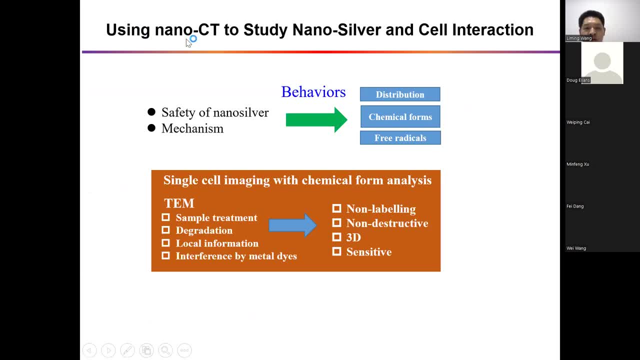 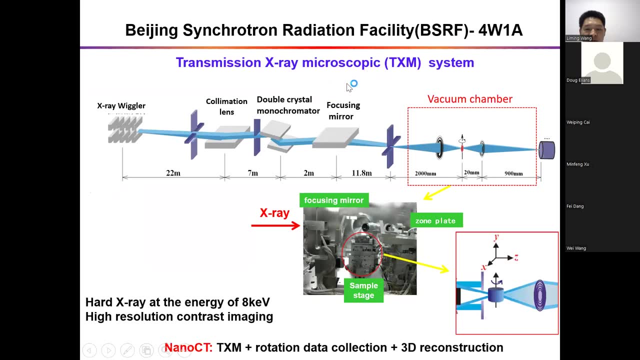 Lianfeng Zhao, PhD. X three bits are you imagine? and the X X three spectroscopy to study the chemical reactions inside the cells. Lianfeng Zhao, PhD. This is the nano city on microscopy. this, this set, sit on working. see x three, go this way and sample. 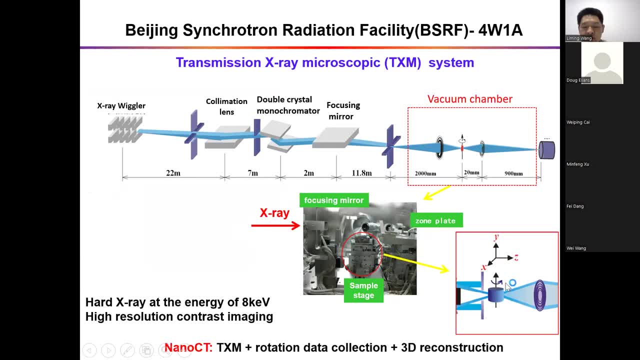 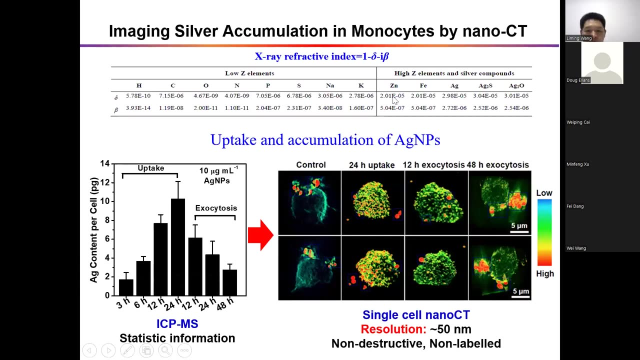 Lianfeng Zhao PhD. Here after the penetration we can get the rotation information and get every construction of sample. get a 3D imagine of the Lianfeng Zhao PhD single sale and we treated the monocytes of sale with the silver particle at different time points and get a sample. then do 3D imagine for the sale particle if I sell that we can see at the beginning and very there are very few. 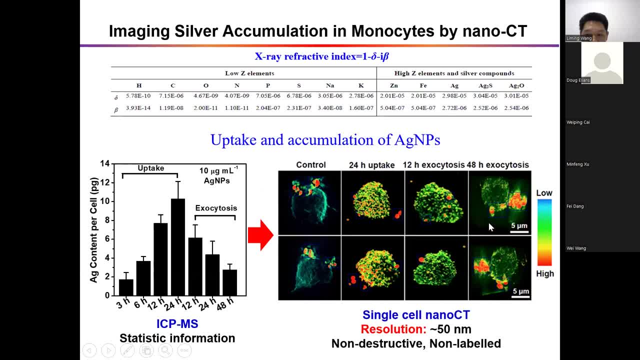 Lianfeng Zhao PhD. Lianfeng Zhao PhD. Here I want to highlight, highlight that they the bread. the red sample is the some go the go the particle to label the sample for images, even though the from several we can see at a 24 hour. there are high accumulation of several particle inside sale. that would time the. 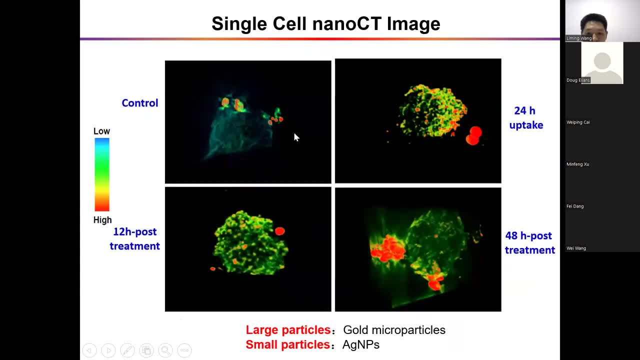 Lianfeng Zhao PhD. The signal decrease with time. Lianfeng Zhao PhD. This is the leak can contract and you can imagine that we'll see the uptake, Lianfeng Zhao PhD, reach the maximum at 24 hours, with time of after uptake of the silver wire degree data and the quality of the best sales. so the thing- and I said sales- decreased based on x ray. imagine. 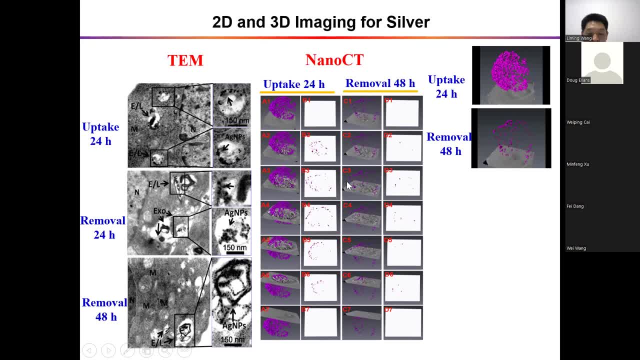 Lianfeng Zhao PhD- And this is also another aspect of the new city- will see the uptake time. this is the remote time. Lianfeng Zhao PhD- The several. Lianfeng Zhao PhD- The several. 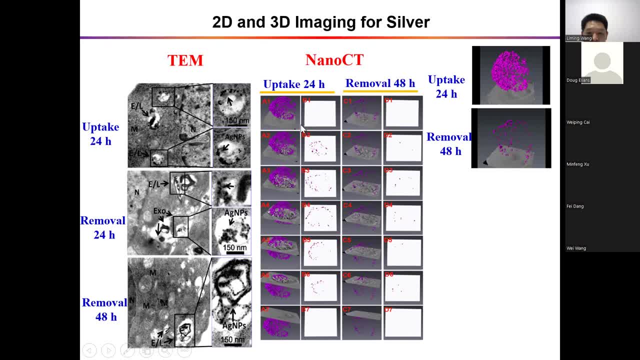 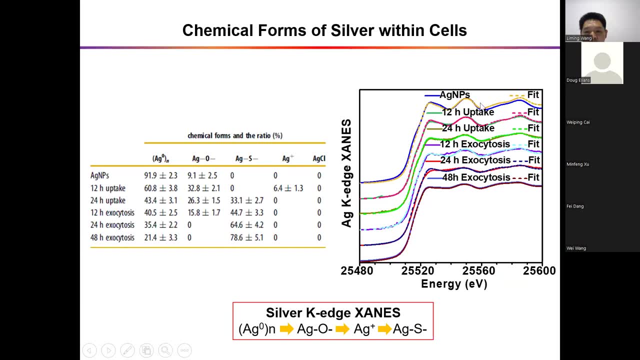 Lianfeng Zhao PhD. The several Lianfeng Zhao PhD signal decrease and then they have a, have a high accumulation. and then what happened to the several? we use the x three absorption. we see the time dependent. 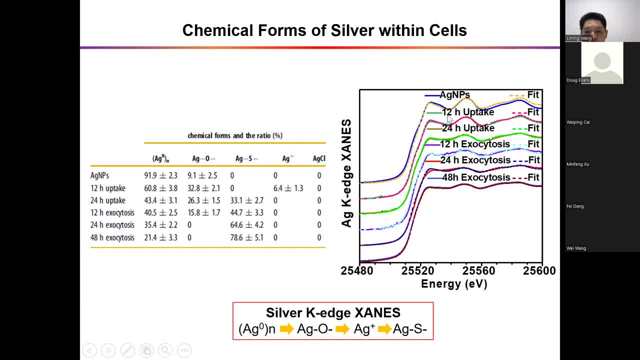 Lianfeng Zhao PhD. On that came the reaction to see double. we can see at the beginning the several remain, the other the elemental, several with time, the several to need to, the several outside and become into a silver irons and several suffice. so other window, monoclonal. 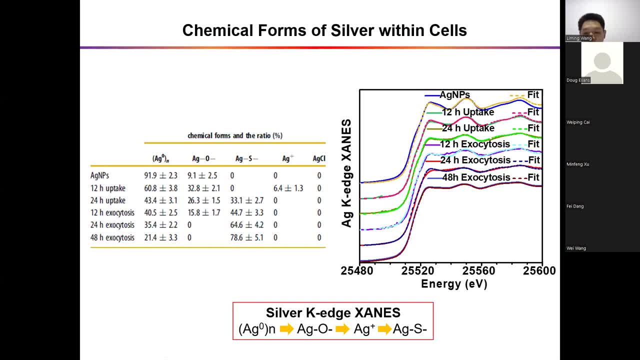 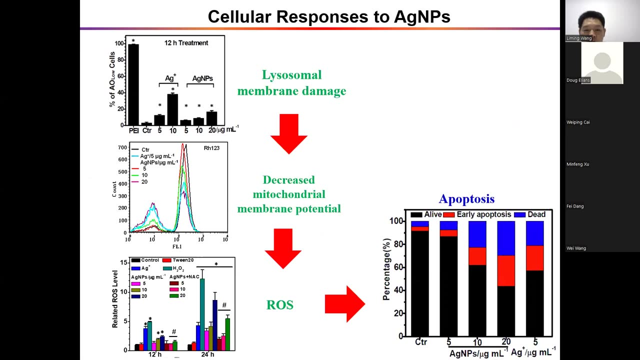 Lianfeng Zhao, PhD. There are some protein and a structure proteins containing the surface, and this is several give of the silver me packet of the proteins and then this self structure and the poor sick. so this work study should the reason why silver particle and in due to sell the toxicity to monocyte of sales by from the chemical aspects. 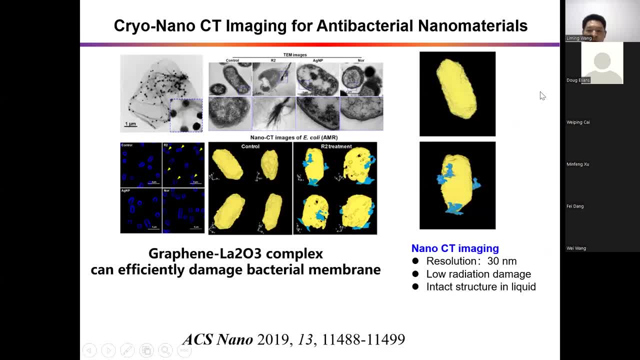 Lianfeng Zhao PhD And, moreover, we can use the Lianfeng Zhao PhD. Nanos city is 30. you may need to study how some nano medicine in a race over the bacteria other window when other window on some bacteria structure is on. 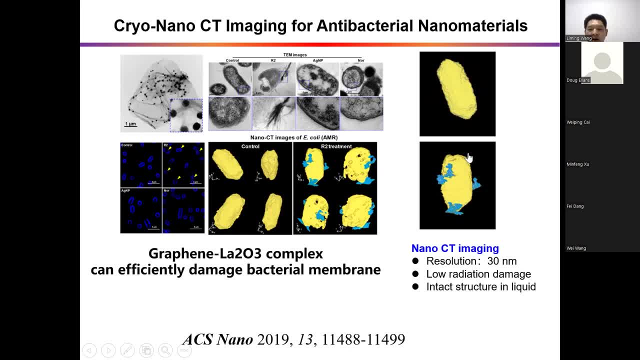 Lianfeng Zhao PhD. A picture can develop a resistance when they are treated that by the anti bag biotics. so we know the material have an advantage to Lianfeng Zhao PhD. To tend to the 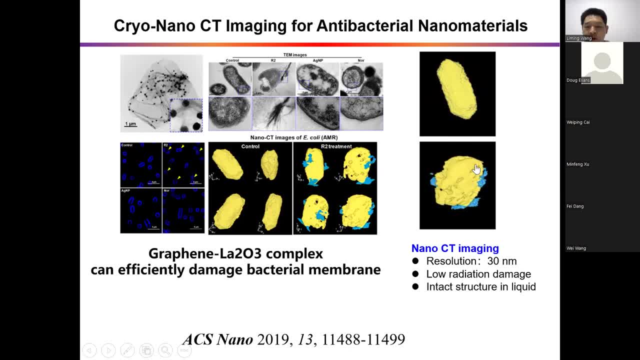 Lianfeng Zhao PhD. The structure of bacteria. so you need to work. we develop on the medicine that they can target to the cell or of the picture, and then your structure. we can, from Nancy, to imagine the Lianfeng Zhao PhD In in our content that will be released and the structure of damage the by the particle- little blue one is the nanoparticle on can direct and attack it as a surface, and then the structures. 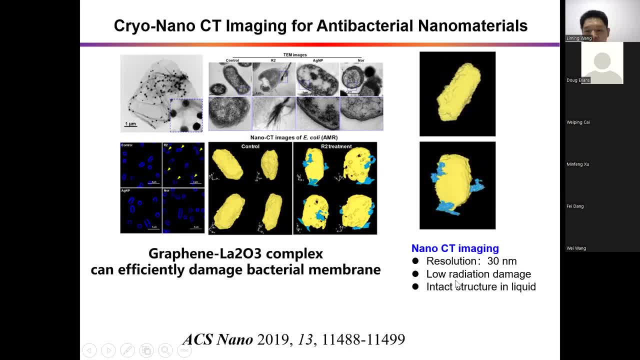 Lianfeng Zhao PhD. So the Lianfeng Zhao PhD Nancy, Lianfeng Zhao PhD, It is you very powerful information about the whole and the material into the cells and the pictures. 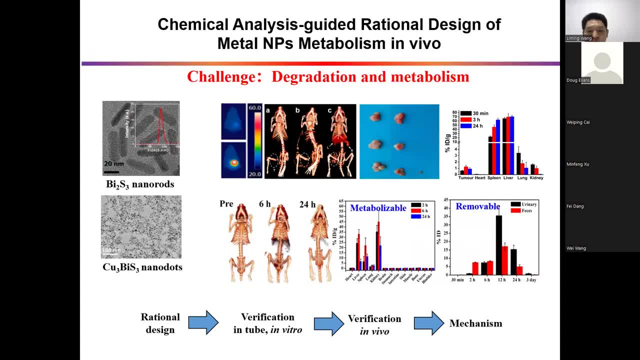 Lianfeng Zhao PhD. Moreover, we can use the an x ray- basically imagine- to study what happened to the sales when the are degraded inside of sales. Lianfeng Zhao PhD. Our previous award show that the business are fat. the nanobot either have to be degraded and committed in the in the NIVA. 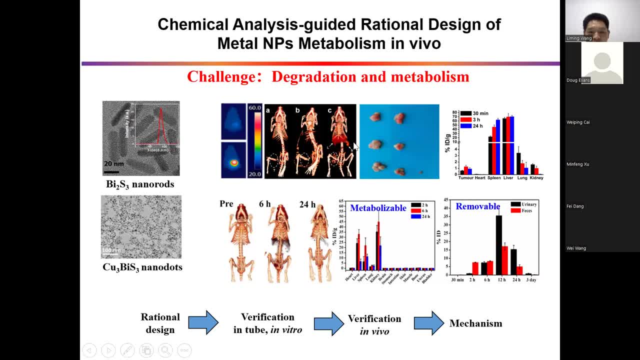 Lianfeng Zhao, PhD For a very long time. so to to help with the degradation on the morning morning for need them. we develop and didn't particle into our small and thoughts. we change the size and get to need the composition of the particle. was found out that these networks can be quickly removed from the NIVA. 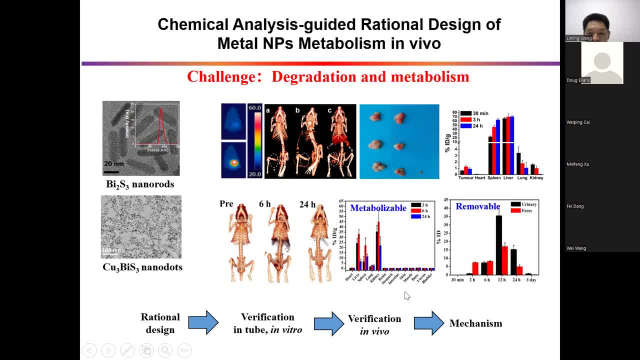 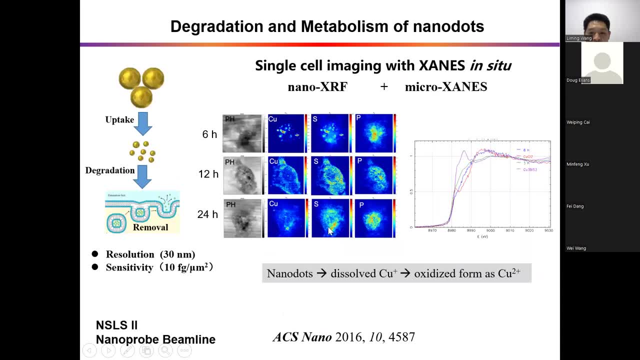 Lianfeng Zhao PhD. So the what is the chemical reaction? and then making them to study the mechanism. we use the x three Lianfeng Zhao PhD. absorption to study. Lianfeng Zhao PhD, Time depends that chemical reaction inside the cells and in some environment and we expose the sales to these and then then dots was founded that at the beginning, that then the particle and contain the Cooper and the 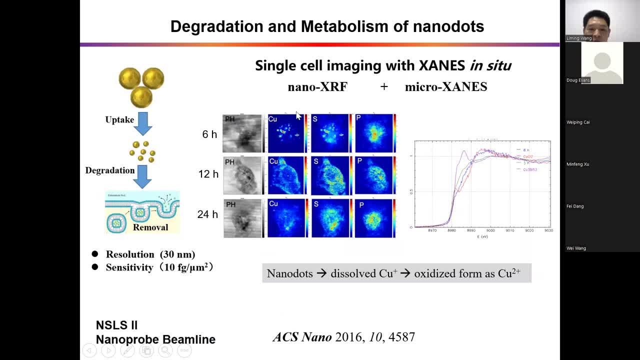 Lianfeng Zhao PhD piece mirth. so we use a Cooper, for example. fun at the beginning. the Cooper either aggregated inside the cells, that such as other, the Lianfeng Zhao PhD trickle, the by. 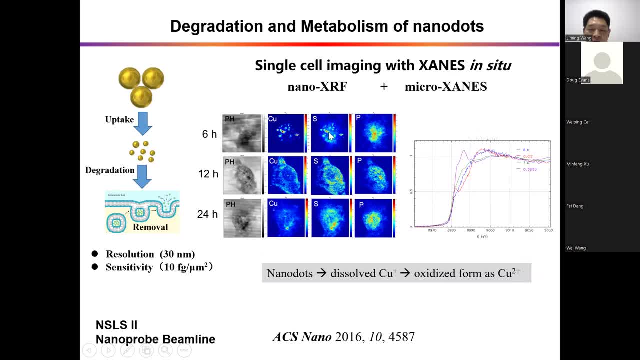 Lianfeng Zhao PhD. verticals and then also they have a good localization with a surface. with time, the, the aggregation thoughts will be disappeared and they are due to be the homogeneous. Lianfeng Zhao PhD For longer time. the Cooper decrease the concentrations inside sales to such in that the Cooper particle inside the element of Cooper in the particle may be removed. the by the sales. and there was a time away. did also detected. 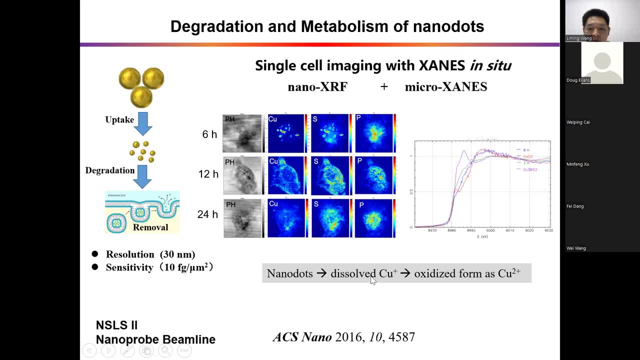 Lianfeng Zhao, PhD. The chemical forms of Cooper we found at the beginning. the Cooper is the venice, the one with time, the why be of the data, from whether to to this, to measure that can. we are in pain, how they then thoughts and 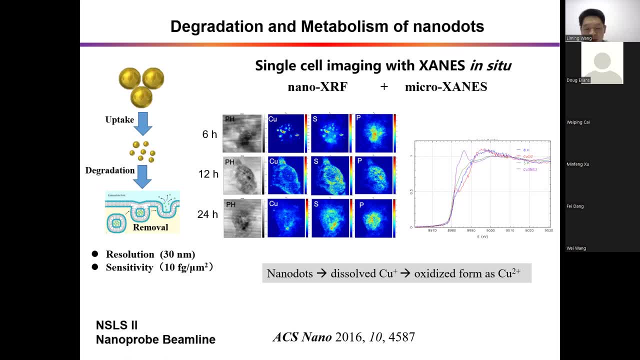 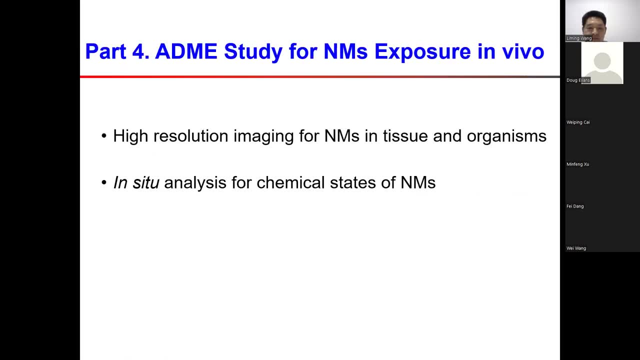 Lianfeng Zhao PhD. What happened to the net doors in chemical ways and you plan how the particle is made the bonnet by by our body. Lianfeng Zhao PhD. And finally, I would like to 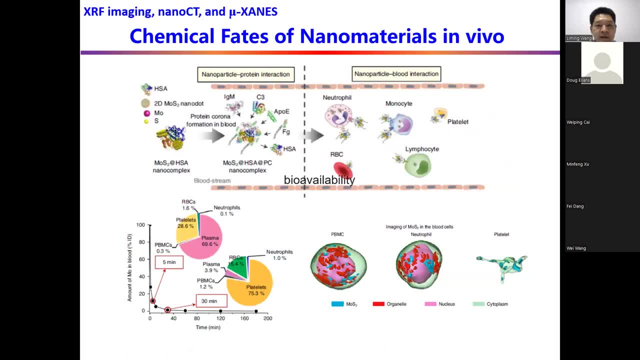 Lianfeng Zhao PhD show how the techniques to study the chemical fits on and mature in vivo. other window: a sun and the material wouldn't the number which inject that you know, but they were talking to some important Lianfeng Zhao PhD. clearance clear. can you read the tissues and such as the nebo and the spleen and spleen. 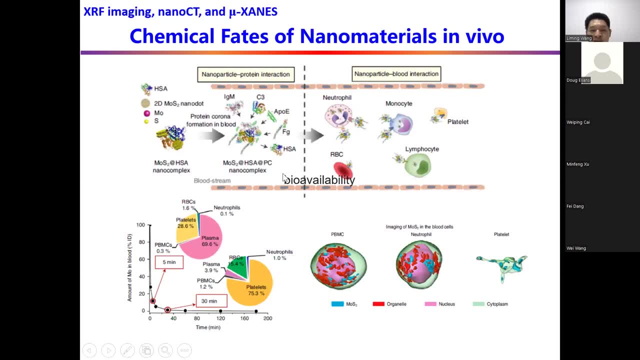 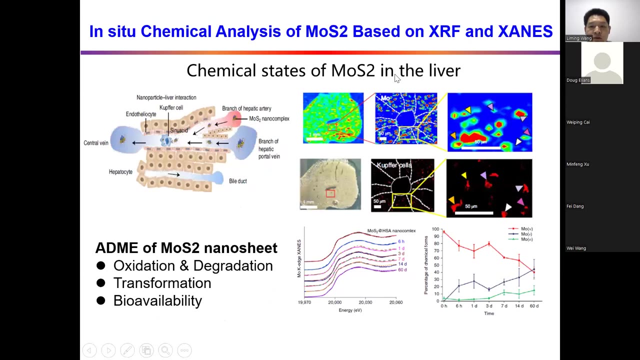 Lianfeng Zhao PhD. So we we use the x ray bits that tiny, such as x three are, x three are a florins, the Lianfeng Zhao PhD Imagine, and the X that's to study the details. and this is one example of how mo s to net particle I and a community in the naval and remove the in the naval. 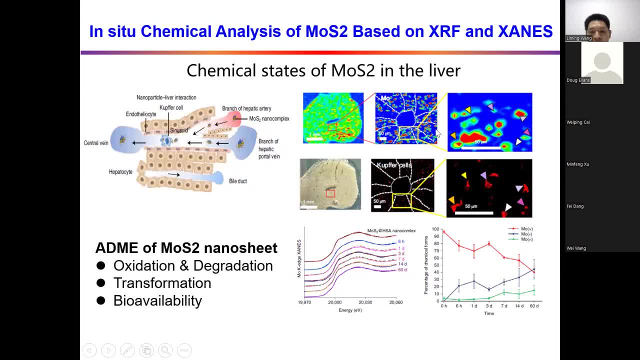 Lianfeng Zhao PhD. We use the x three and when the particle in general in the blood they are quickly go to the level and to the good and evil because the medical particle have the matter mo- Lianfeng Zhao PhD elements. so we use the x three, X after, imagine we can see the distribution of elements of mo in the level. then we the high resolution mode to detect the mo. we found the mo have some spec. 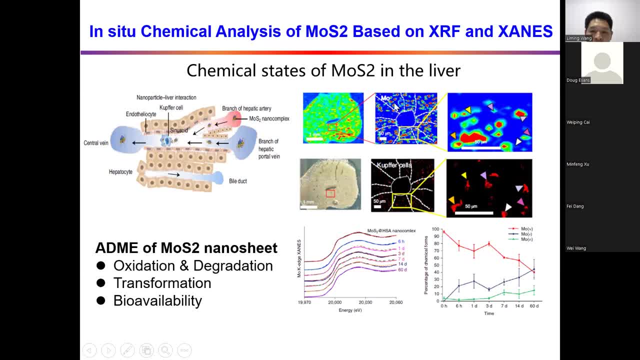 Lianfeng Zhao PhD. Specific or distribution in specific, because sales we use the F on you. Florence on Lianfeng Zhao PhD. immune. Florence to Lianfeng Zhao PhD. detect the, the macrophage inside the level, finding that mo have a very high localization of the Cooper fair. this is a macro, a kind of macrophage itself. so they have very high localization at the beginning. with time we found out that distribution code, distribution of 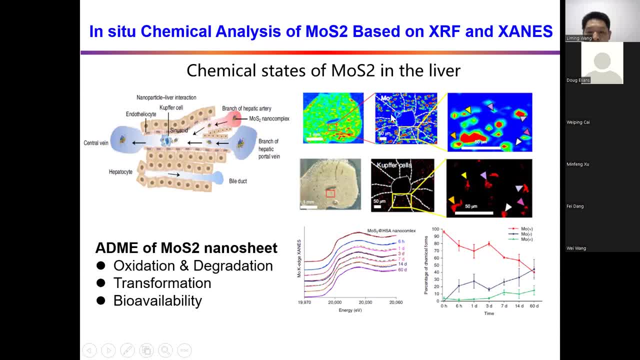 Lianfeng Zhao PhD Macrophage it will be to appear. they will have more to to build on with the newer sales. so what happened to the mo Lianfeng Zhao PhD? As to nanomaterials, we use the 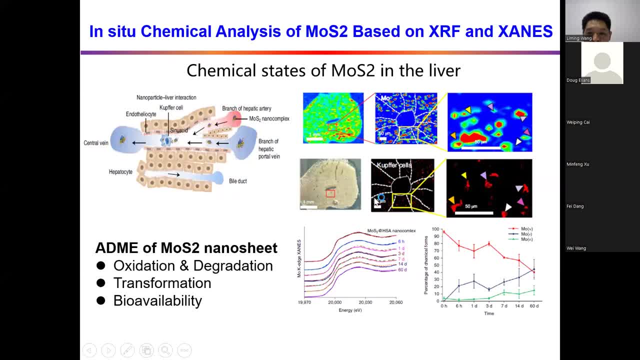 Lianfeng Zhao PhD. That x, three assumptions. but if you had what happened to the level with time at the beginning, we found that the mo have a balance of four. with more time they balance the way we change the violence of mo balances five and six. 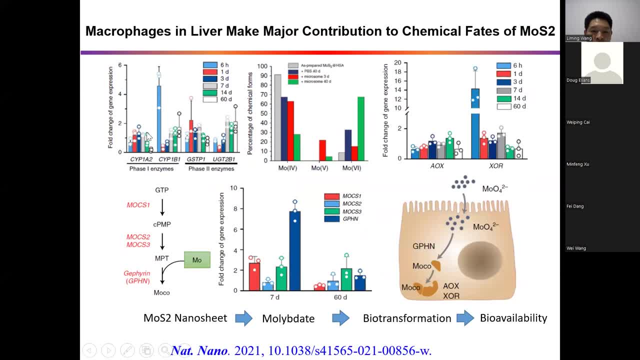 Lianfeng Zhao PhD And other window, the mo, elements in the important for the and then the, and then mo, and then Lianfeng Zhao PhD. In fact, the level, the evil Lianfeng Zhao PhD For them a or X or X, or are there are two kinds of? 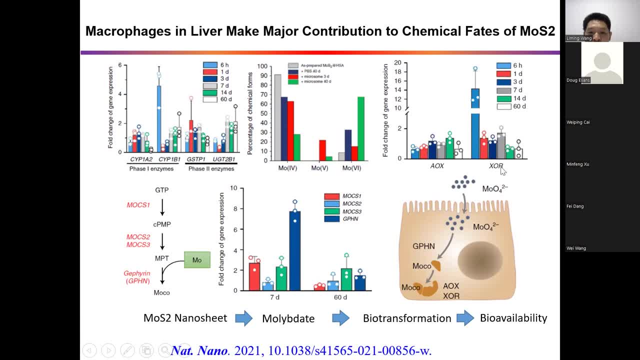 Lianfeng Zhao PhD, Metabolism, and then and link including mo elements. so we found that the after inclusion to the net particle the naval rdp Lianfeng Zhao PhD. Mr. level of the. 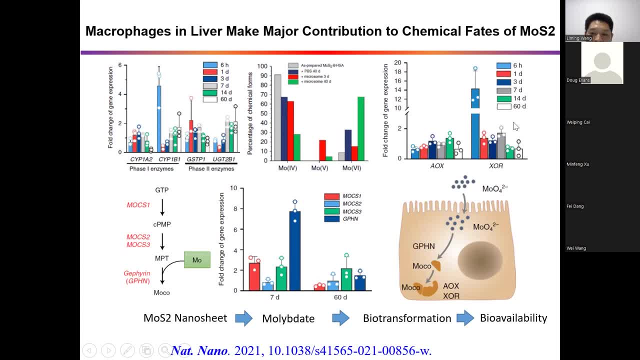 Lianfeng Zhao PhD. The two molecules increase with time to suggest that Lianfeng Zhao PhD, An mo maybe trying to form to some about valuable molecule nurse. Lianfeng Zhao PhD These two and then have some. 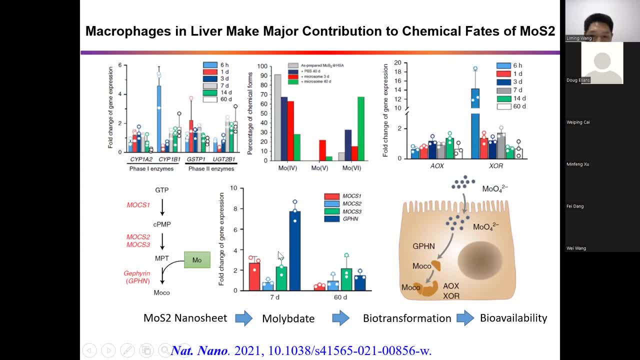 Lianfeng Zhao, PhD, mo cool factors. so we, based on this monoclonal biology evidence and x three based on evidence, we can see that when mo s to Nana sheets were injecting the blood, the good to the level then they 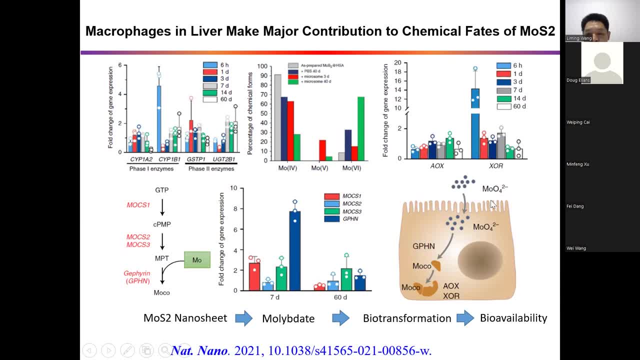 Lianfeng Zhao PhD Are be multiple in them and you would be good data that into mo mo o for these kind of high balance can form. then this kind of form, me kind of form mo factors into the Lianfeng Zhao PhD mo than, and then there will be. 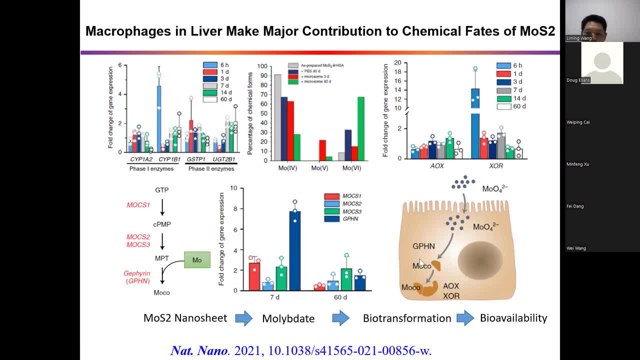 Lianfeng Zhao PhD, The the the one new ways for the degradation and the transformation of many materials. Lianfeng Zhao PhD Is a new. Lianfeng Zhao PhD- face. Lianfeng Zhao PhD- New way for the face of nanometer. they can become a part of the monoclonal after the degradation and the kind of form transforms. 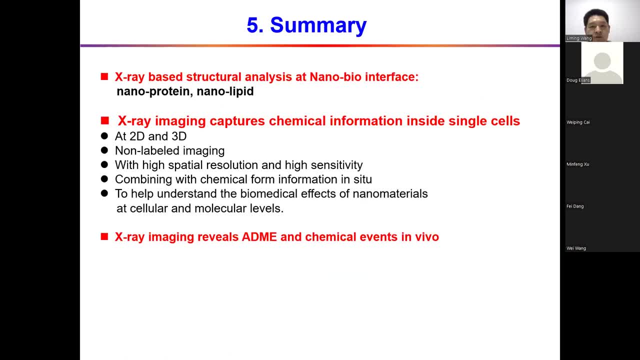 Lianfeng Zhao PhD. So these worker on. so we're good. to the summary. we use the x three beats, the Lianfeng Zhao PhD techniques to study how many material integrators with our biology system at a monoclonal level, senior level and the 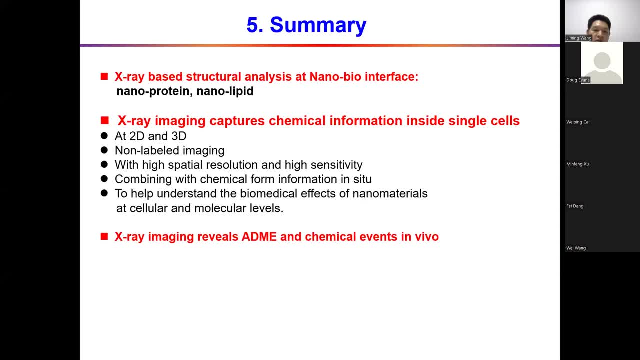 Lianfeng Zhao PhD, The tissue and the whole body level, the techniques that can show on very important structure information. to focus on what can detect the, the protein signal structure, can shoot on, can shoot the nippy, the structure. and Lianfeng Zhao PhD, And the, the invasion can show what happened to nano biology at the beginning, you at the beginning. 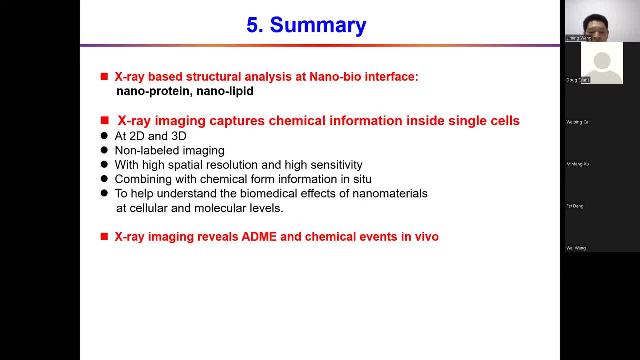 Lianfeng Zhao PhD. In the event Lianfeng Zhao PhD. Later, when the nanoparticle go inside the cells, there are some kind of physical and chemical reactions to nanomaterials. for example, Simon redraws, can I see kinetic connective and degradation and the transformation and 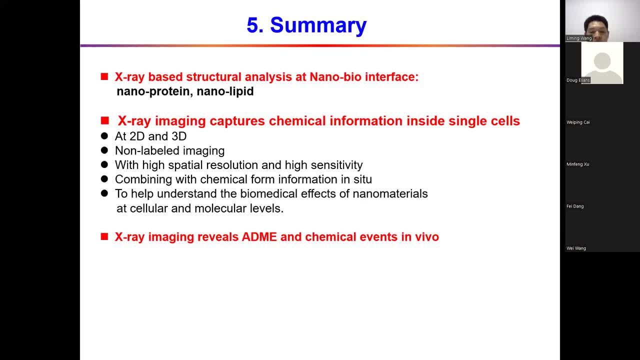 Lianfeng Zhao PhD. Bell. Lianfeng Zhao PhD. Bell transformations during the chemical reactions. x three based on imaging, and Lianfeng Zhao PhD and Lianfeng Zhao PhD And the x three absorption based on spectroscopy, can detect a. 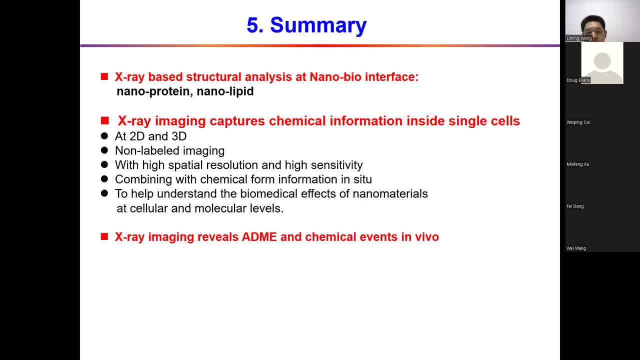 Lianfeng Zhao PhD. chemical reaction in situ, the, the in situ where Lianfeng Zhao PhD. Well, you explain on the chemical fits of the particles inside the cells and in the tissue and in the whole body. so we think of this on combined of x three, imagine, and then liquid environment. 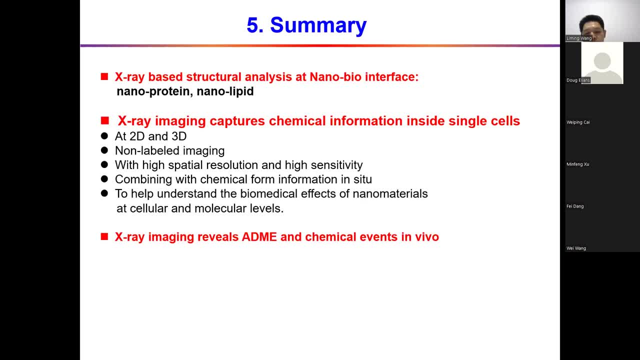 Lianfeng Zhao PhD. And then: Lianfeng Zhao PhD, Bio interface techniques can shoot very detailed information. Lianfeng Zhao PhD For nanomaterial. you can read it with our body and the system. these are also powerful for the developer of nanomedicine in the future and in the future, not only for the on the performance of nanomaterials, but also for the 70 evaluation. 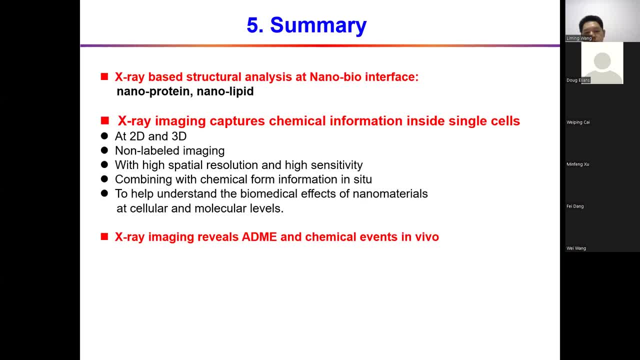 Lianfeng Zhao PhD And Lianfeng Zhao PhD. Moreover, the on this techniques are not only Lianfeng Zhao PhD, powerful for the nano and bio interaction. they are worth very powerful for the application in the environment, science, science and they can be also use. study the particles. they hit his particles in in the air pollution. we also do some work to study how the matters are distributed. you know particles. 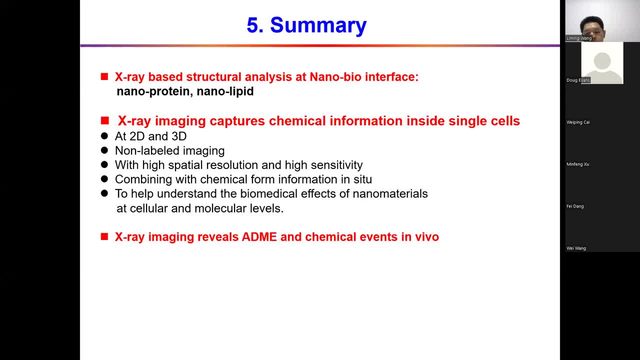 Lianfeng Zhao PhD. You know micro meter said particles. to know how the particle, Lianfeng Zhao PhD induce the opposite of the data with stress and toxic to sales. so I think on this, Lianfeng Zhao PhD leader on powerful techniques, that will be helpful for an hour study little about nano biology, but also for 10 sentences: the in environmental science. 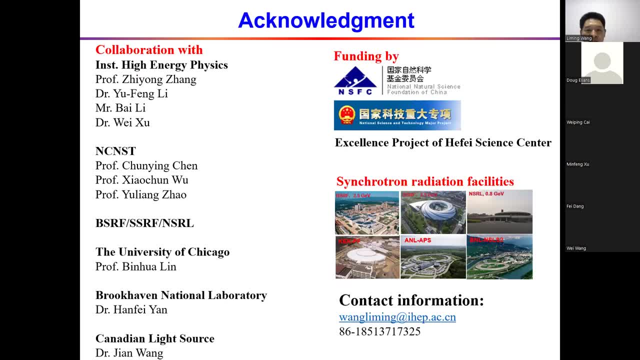 Lianfeng Zhao PhD And Lianfeng Zhao PhD And- and I would like to thank you- my collaboration with my calling in institute of our allergy nano national Center for nanoscience and technology. and Professor. 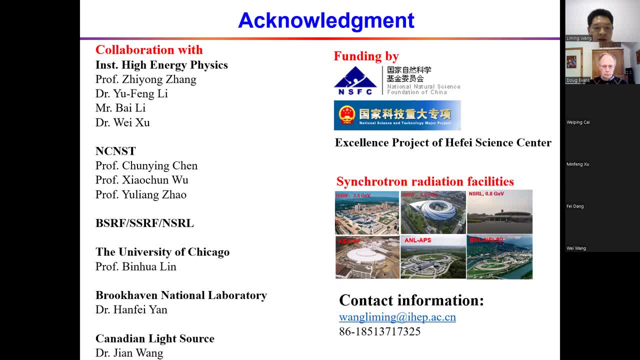 Lianfeng Zhao, PhD, A train train, prefer the shopping mall and prefer union job. and I also like to thank you my collaboration with the thing called radiation facility in China and the from us and Canada. Lianfeng Zhao PhD, Canada, the provider. very. 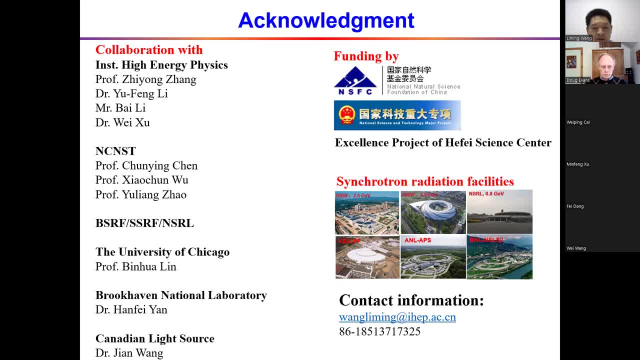 Lianfeng Zhao PhD. Plenty, plenty on beam time and a very instructive on Lianfeng Zhao PhD, Powerful techniques for study, and so I would like some funding from channel on channel and the whole free Center centers. I. 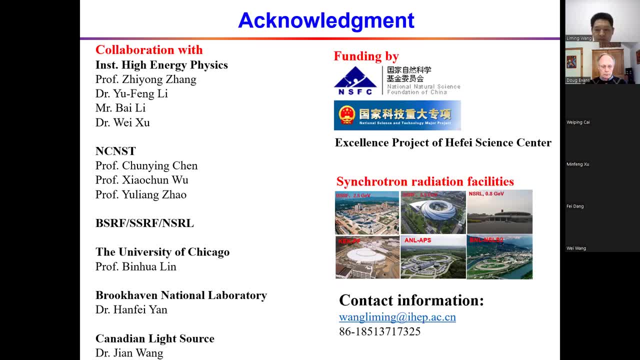 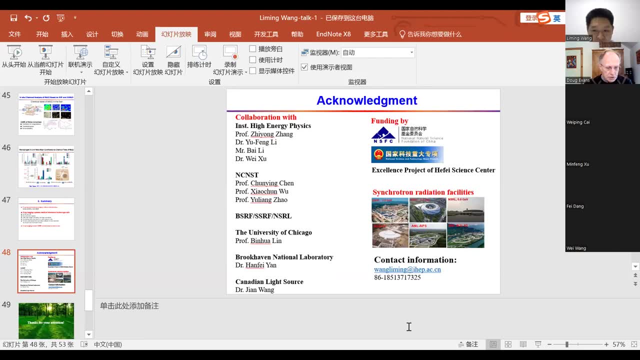 Lianfeng Zhao PhD. Finally, I will thank you for your attentions. Lianfeng Zhao PhD. Thank you very much, Professor wall. that was an excellent introduction to Lianfeng Zhao PhD, What obviously is a very complex biological systems in which you're working. 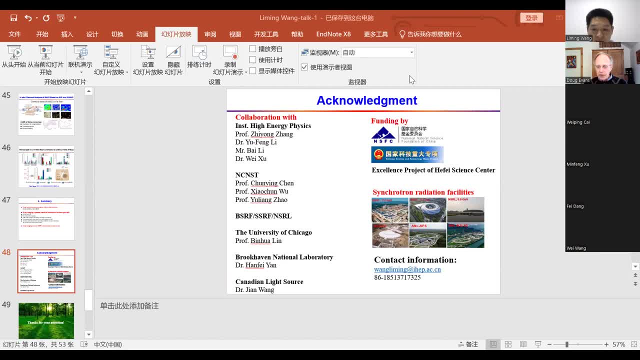 Lianfeng Zhao PhD. I would now invite people to ask questions. I would also invite you to turn on your cameras, if you wish, so that we can see who's actually asking the questions- part of the purpose of these. 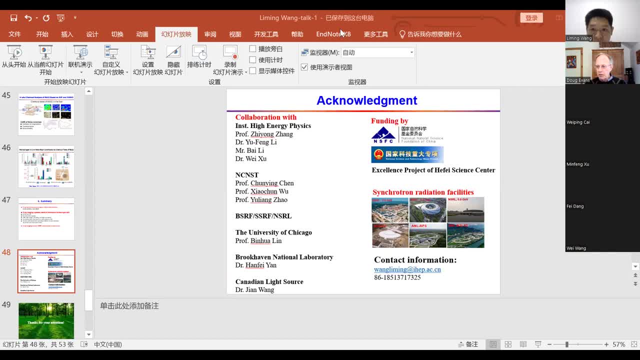 Lianfeng Zhao PhD lectures. Lianfeng Zhao PhD And Lianfeng Zhao PhD lecture series is for you to get the opportunity to perhaps get to know people around the world working in other areas. so you can ask your questions either using the chat function. 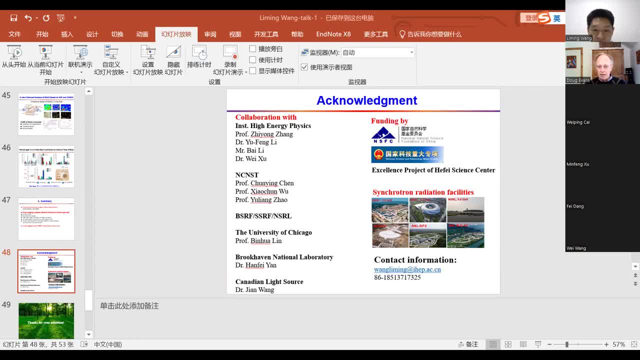 Lianfeng Zhao PhD, Or you can open your microphone and I see that we have a question from Ian Oliver in the UK who asks: your data shows that the nano particles can penetrate cells. once they have penetrated, cells really tend to remain inside them. 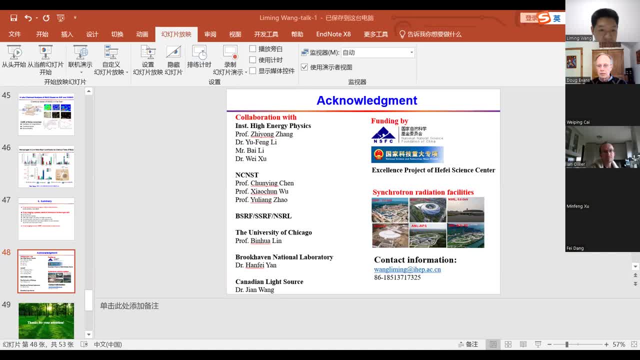 Lianfeng Zhao PhD or are they Lianfeng Zhao PhD, Still mobile and reactive? Lianfeng Zhao PhD And thank you Lianfeng Zhao PhD, Professor events. thank you for the question. 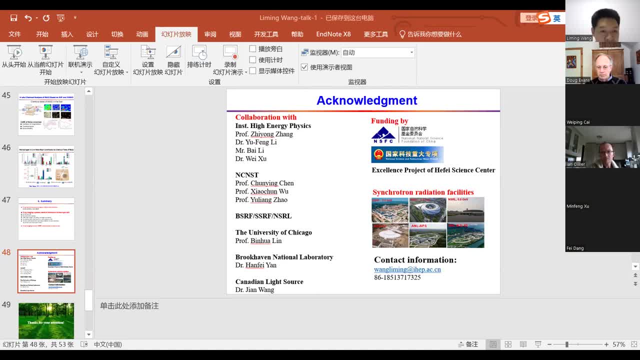 Lianfeng Zhao PhD. um see them in a particle computers? Lianfeng Zhao PhD. Oh, it's a very good questions. um Lianfeng Zhao PhD. And it depends on the cell type and then the, then the type of nanomaterials, for example. 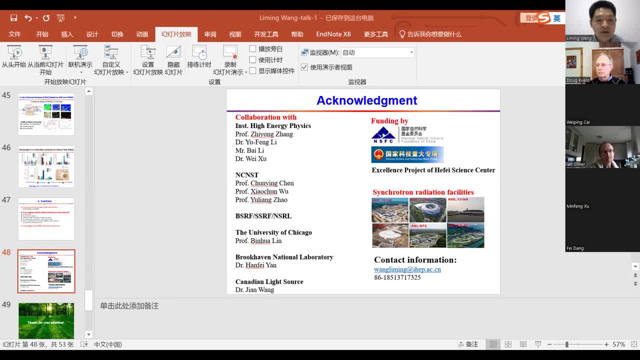 Lianfeng Zhao PhD and other Lianfeng Zhao PhD. Other Lianfeng Zhao PhD. Other Lianfeng Zhao PhD. For some carbon nanomaterials and when the intake of when they are uptick in the by the macro phage milk time they are remain the in the sales. for some matter, particles, the chemical react reactive. for that, for example, for Cooper and several the, they were being moved. 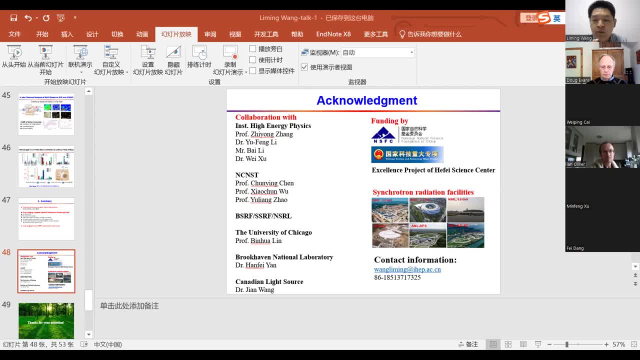 Lianfeng Zhao PhD, Jose, and they will be degraded, they will be removed. Lianfeng Zhao PhD, by the Lianfeng Zhao PhD cells and, moreover, some particle may be trying to form from one place to another. one of our previous work to show that if we could see the particle with some 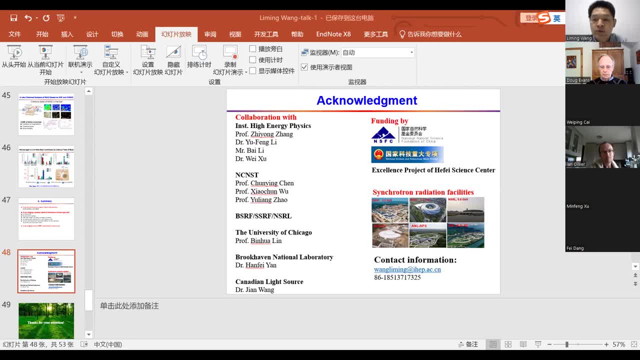 Lianfeng Zhao PhD certificate and monoclonal go. we could do that. the golden road with the certificates in the monoclonal, such as the ctap, did monoclonal condemned the memory of the lesson, then in this case, the 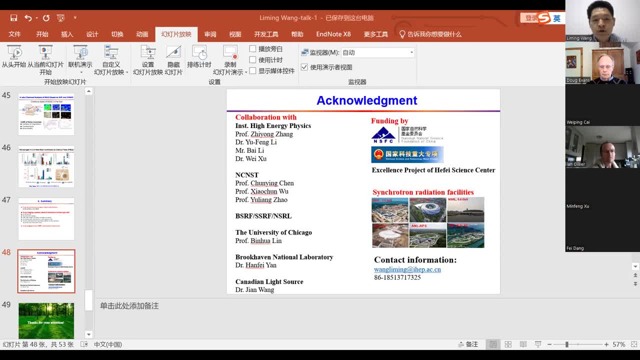 Lianfeng Zhao PhD, ctap. good night. or the me. Lianfeng Zhao PhD, me trying to. for. Lianfeng Zhao PhD, From. and some lesson to make. the country are so. this particle moves, move the from one place to another. inside sales. so you so? the answer is that you depend on the cell type and the material tech. thank you for the question. 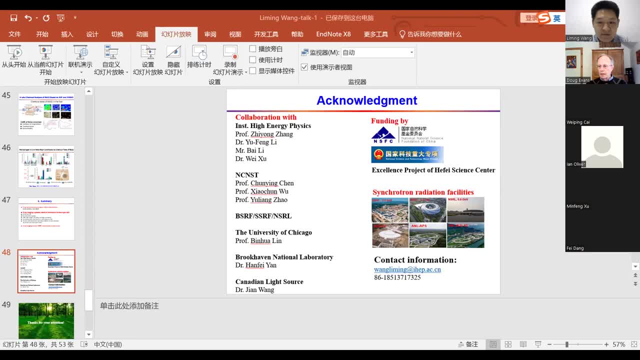 David Sloan- Other questions for our speaker today. David Sloan- Maybe while you're thinking about that, let me ask you one. David Sloan- living David Sloan- A lot of what you've shown us today is experimental work where you can. 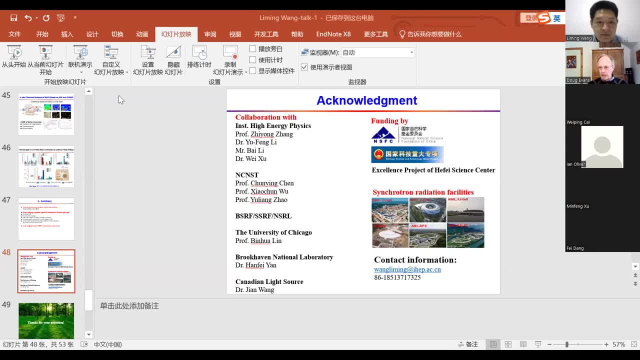 David Sloan- You know, prepare your sample and then directly take it to the facility. but if we think about extending this to more environmental type samples, David Sloan- Does sample preservation become an issue? David Sloan- In other words, how long would you? 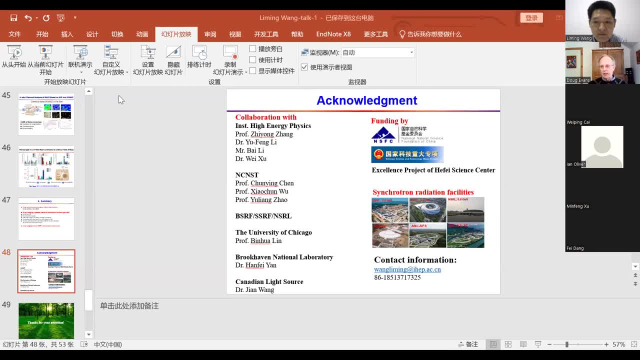 David Sloan- Like, how long could you wait before you analyze a sample, David Sloan-? And given the- you know limited number of facilities that have the synchrotron type facilities that you're talking about, David Sloan- You know, how does that play into ability to analyze real world samples? 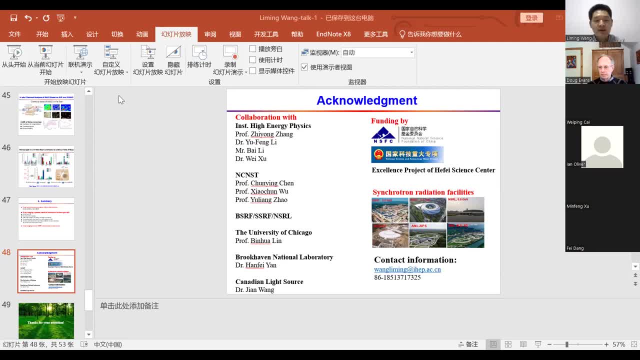 Lianfeng Zhao PhD. yeah, very good question and prefer that you event um Lianfeng Zhao PhD And for the other one, know the beam time for synchronous relation, either on pressure? Lianfeng Zhao PhD And what for? for different: the sample will have different way to prepare for x ray based on the quits. we didn't. the technical reaction is not involved. we can do them to them. your time. yes, we can take a sample and then prepare the new. nip it on the trough surface. that we can do at once. we need to care about the 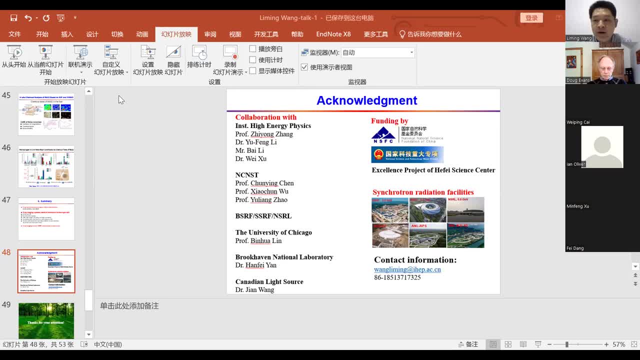 Lianfeng Zhao PhD. The Lianfeng Zhao PhD For example, for some cell and then elementary interactions- it is actually a Chinese for them before good for good. not a lot interact with on sales go to the inert. so in maybe not the problem. we can if we incubate the sales with a particle. 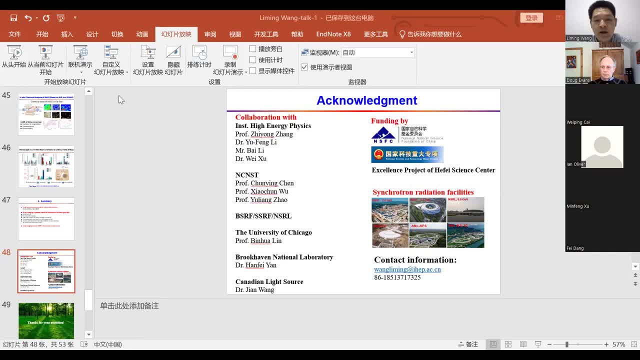 Lianfeng Zhao PhD, And then try to them and then store them in the air free on tubes or after a Lianfeng Zhao PhD, nurse, okay, and then we take a sample to for y three, imagine, and the on detection. that even the problem, but for several is also questions- is actually the question, because they have all either chemical reactions and 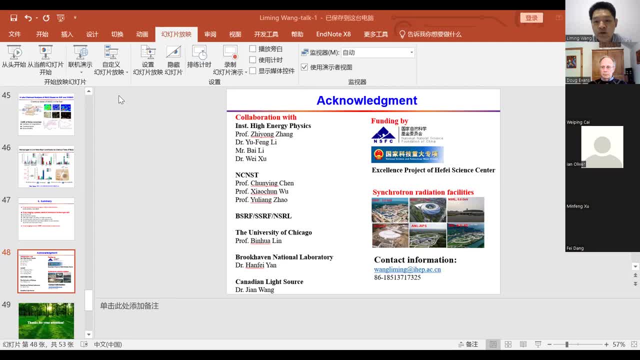 Lianfeng Zhao PhD. yeah, we, we just the try our best to shorten the time between our experimental time and a sample prepare time, Lianfeng Zhao PhD, Because with longer time the silver me interact with the monoclonal and some things. actually we, 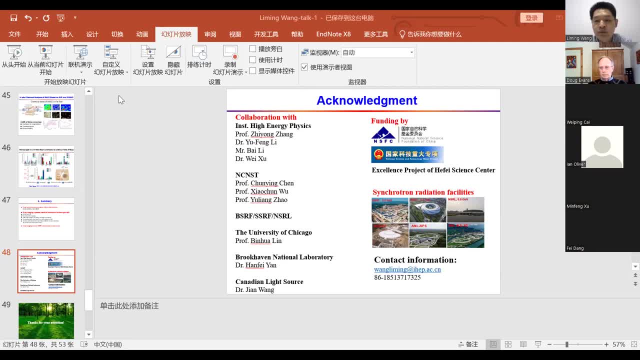 Lianfeng Zhao PhD. yeah, one better way that we try the samples and then put them in the air free system and the in core system. and in the future, we, we want to do some improvement. for example, we, we want to. 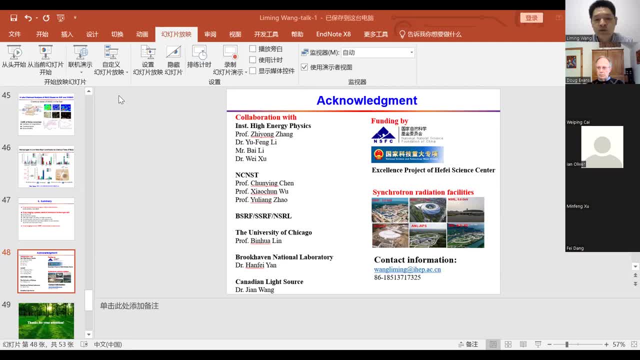 Lianfeng Zhao PhD. try to develop some system- Lianfeng Zhao PhD, To quickly try the samples, maybe in several hours or several minutes, to try the samples. that either. Lianfeng Zhao PhD, A better way to to get the viewer information. 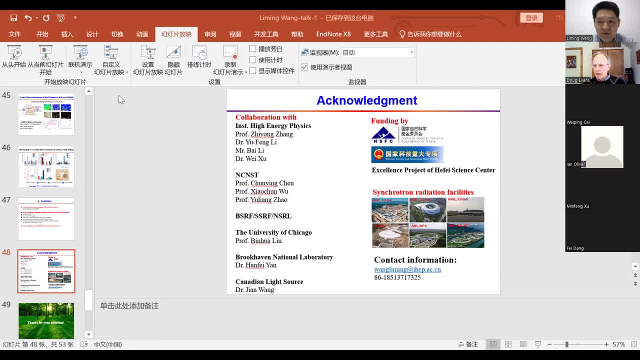 Lianfeng Zhao PhD. Thank you, thank you, um again. i'll invite other questions, but if there's no question at the moment, I have another one for you, Lianfeng Zhao PhD. So any questions for living. 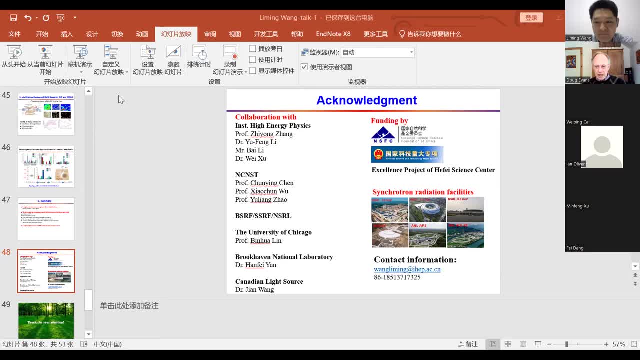 yeah, Lianfeng Zhao PhD. If not? so this actually follows a little bit on my last question. and when we get into real world samples- so, for example, some of your work on inflammation or drug transfer and so on- and in the real world? 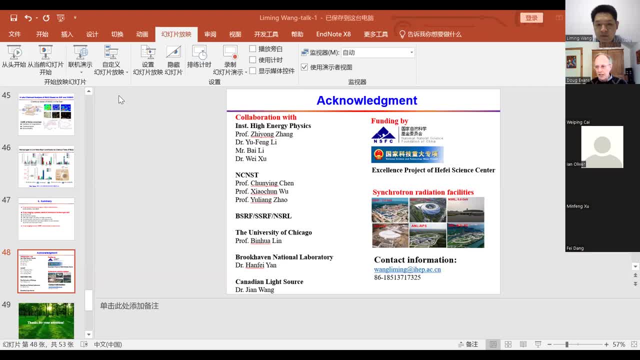 Lianfeng Zhao PhD. People might have other sources of nanoparticles that. might Lianfeng Zhao PhD interfere, I guess I would say, with some of the signals and- and I guess my question is really about the complexity of samples and how that affects your ability to separate out specific signals for some of the nanoparticles that you're looking for. 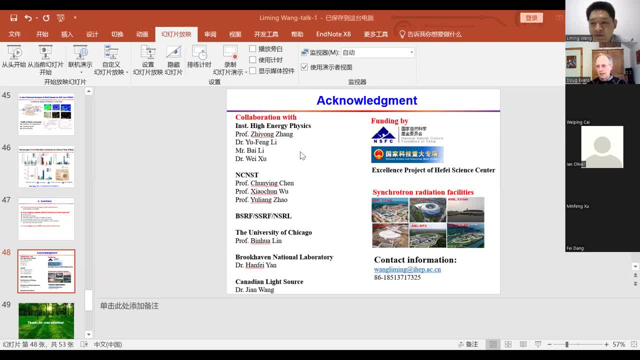 Lianfeng Zhao PhD. I didn't master you question about nanoplastics. Lianfeng Zhao PhD. yeah, not about nanoplastics, but about so, for example, Lianfeng Zhao PhD, If you're interested in: 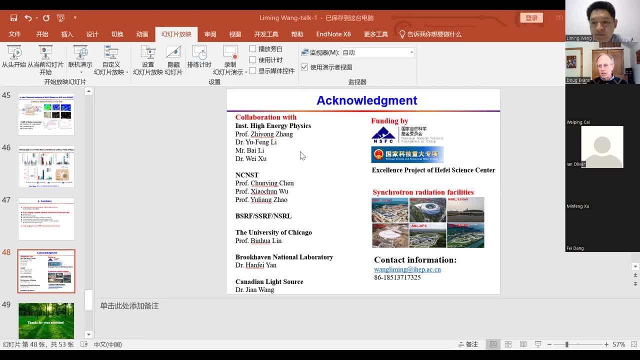 Lianfeng Zhao PhD. Looking at the effect of, say, Lianfeng Zhao PhD, A drug delivery, that you're using a nano particle carrier for right, yeah, and in your work where you, where you have that in a sort of isolated system. 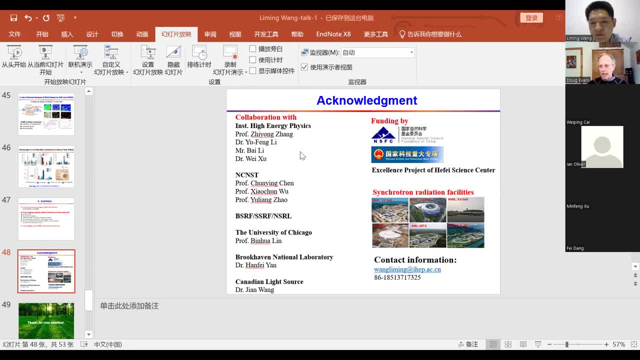 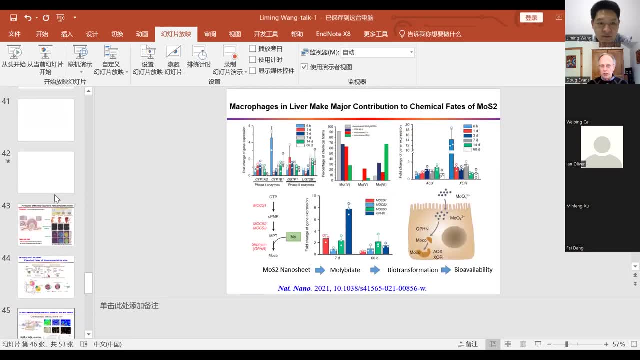 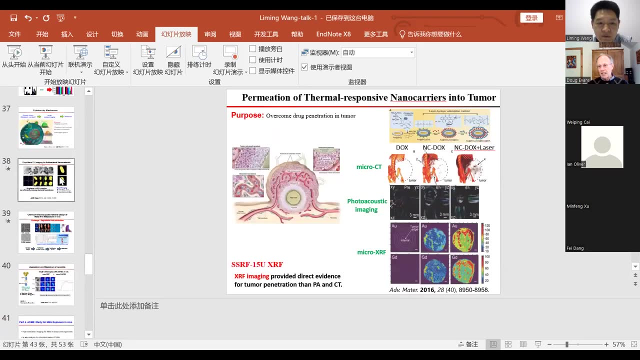 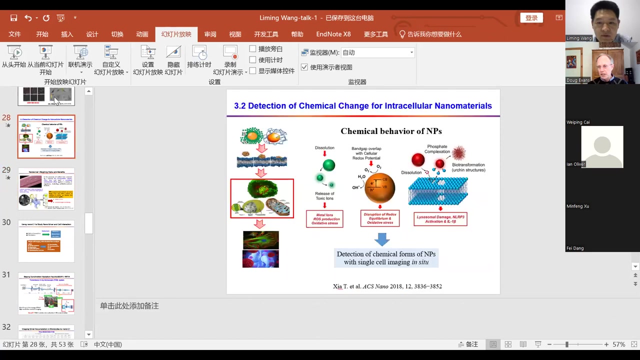 Lianfeng Zhao PhD, You can see very clearly the signals and watch the transformation or the the translocation of the drug, that sort of thing, but in a real world, individual, where you know if i'm taking that drug. Lianfeng Zhao PhD, let's say it's a platinum drug or something like that, but I might have other sources of materials that might interfere with those signals that you're seeing. 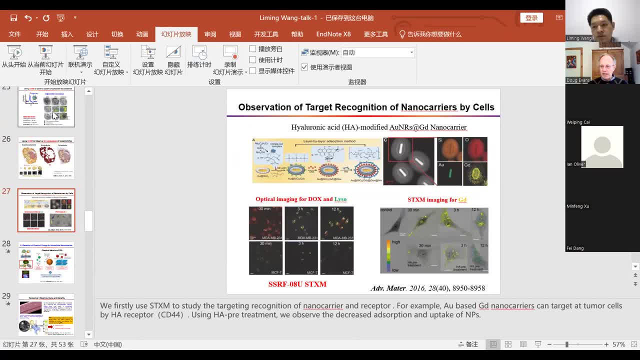 Lianfeng Zhao PhD, And so i'm just wondering about how complex samples affect your ability to actually trace some of these processes that you're. you're watching Lianfeng Zhao PhD, Oh yeah, um, Lianfeng Zhao PhD. It actually in the signal pathway is too complex and 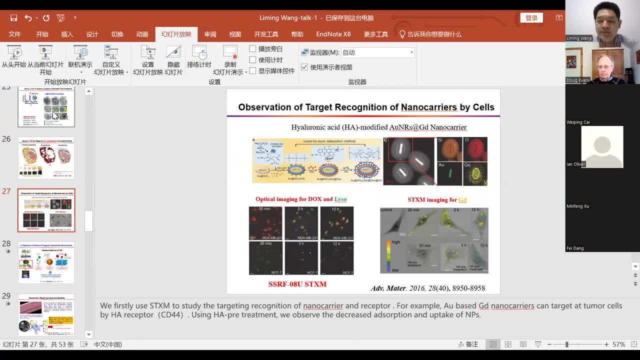 Lianfeng Zhao PhD, But I think either also Lianfeng Zhao PhD In fit on how to say it, may works. I think I either works for some signal pathway. Lianfeng Zhao PhD, It for example on: 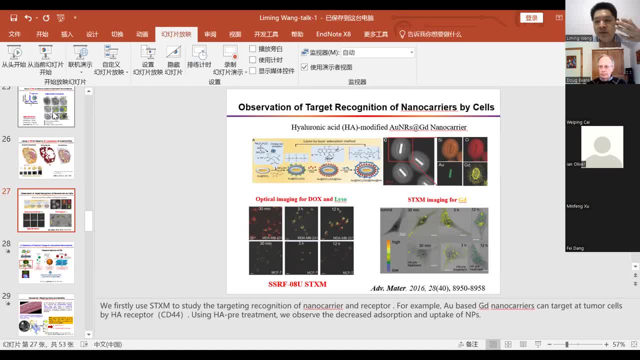 Lianfeng Zhao PhD, um, your your name, some then particle maybe up, taken by micro feeds by some cell receptors. yes, you need the case. you want to verify, would you? would you kind of receptor on are involved in the uptick and 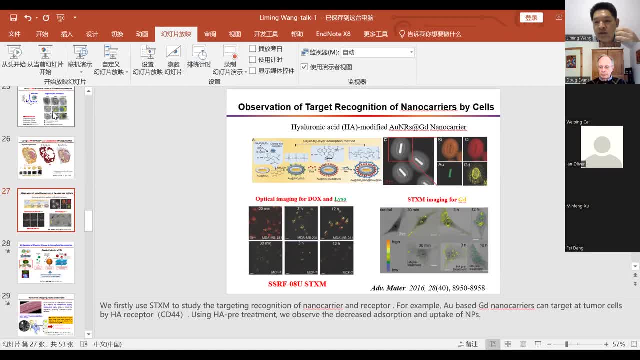 Lianfeng Zhao PhD. So you want to study, if he wants that, that you can use some anybody- and some small, small molecular inhibitors to to block or block the surface or micro feeds. then you can see very less of the up up to our distribution of the metal elements inside of the tissue micro feed. 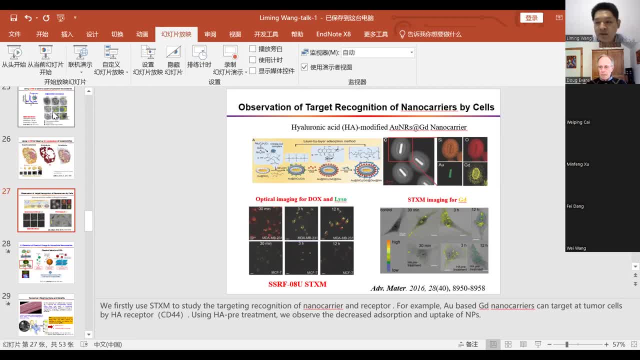 Lianfeng Zhao PhD. Sorry, i'm not sure i'm Lianfeng Zhao PhD. I can steer on another way. is that and some? there's a miracle company, developer or elements, the earth elements based anybody and how see? 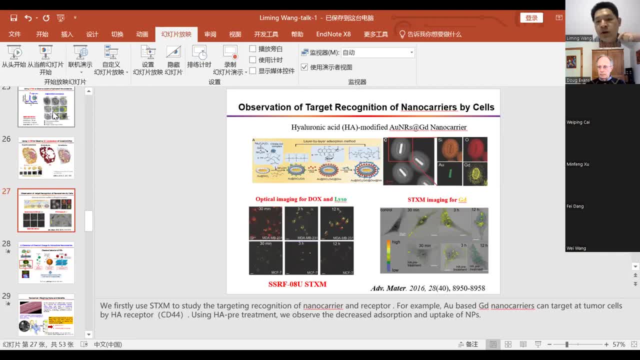 Lianfeng Zhao PhD, You that anybody can use some of elements. you can use anybody to block. block the specific monoclonal in the techie, the sales. you can, Lianfeng Zhao PhD, Not only see the particle elements but also see the earth, chapter the receptors to see whether they are colloquial addition or or other. on the collaboration, I think the key is a very interesting to see what happened to sell in vivo. 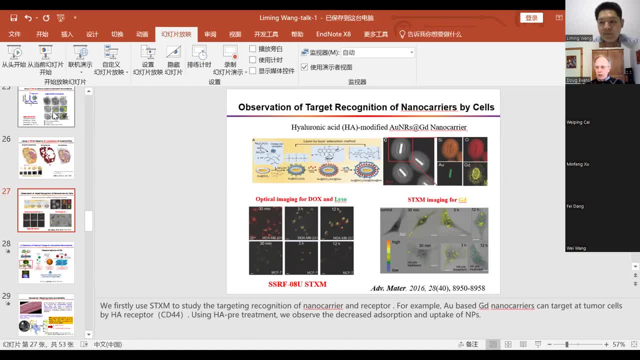 Lianfeng Zhao PhD. yeah, makes a lot of sense. Okay, thank you, Lianfeng Zhao PhD. So other questions for a speaker. is your last chance to get in and have your questions answered? Lianfeng Zhao PhD. So I have a question from pain. thanks for excellent report and I wonder to know if synchrotron radiation technology could be used to observe the interaction. 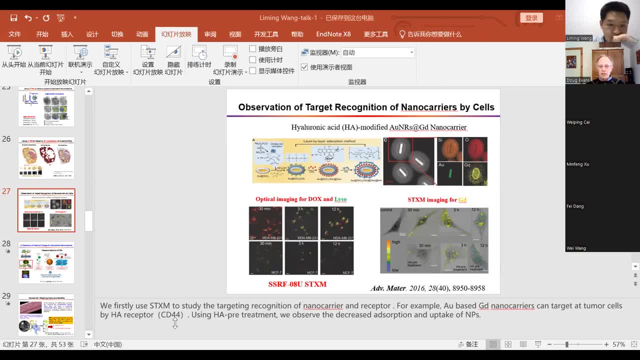 Lianfeng Zhao PhD, Between proteins and nano particles on bacterial cell membranes and how to determine which protein on the membrane is bound to the nano particle. yeah, Lianfeng Zhao PhD. Well, thank you for the question. actually, I have a question. I have a question about the. 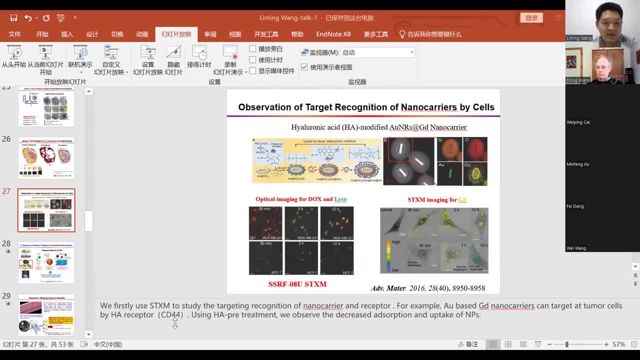 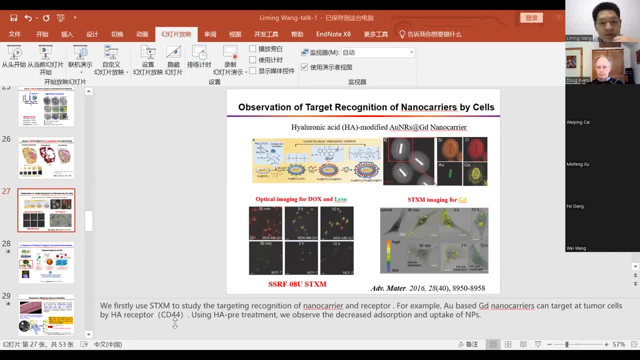 Lianfeng Zhao PhD. special resolution of the x ray imagines. yes, Lianfeng Zhao PhD, If the Lianfeng Zhao PhD, The Lianfeng Zhao PhD, The, the, the. 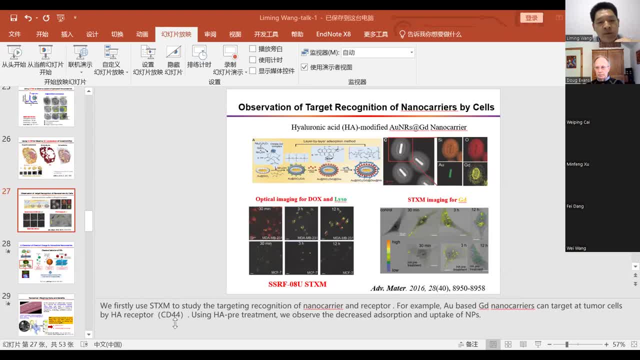 Lianfeng Zhao PhD. The native on the. Lianfeng Zhao PhD, The the best resolution now, maybe rated to two nanometer resolution. I think either possible to detect the, a single protein on the pictures and other. I mentioned that on us. us company can. we can buy some. 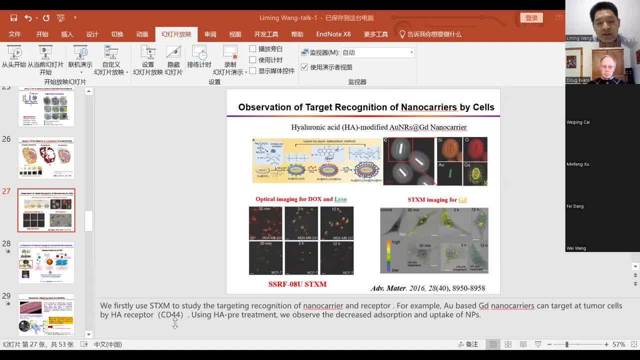 Lianfeng Zhao PhD. Real earth element modify the anybody and that anybody can talk it to the surface or back to us. Lianfeng Zhao PhD. So Lianfeng Zhao PhD, First. 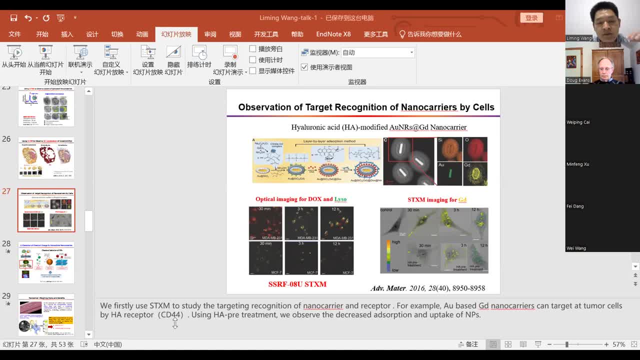 Lianfeng Zhao PhD. You label the surface that with the real earth elements. then you use your metronome particle interactive with the Lianfeng Zhao PhD bacterial surface to see whether they have a good and have a good call in the condition. you will have a good clinic and they can see the protein, maybe the target, the proteins. of course, an extra piece of techniques that can show that the director evidence for their interaction. I think another way you can use some 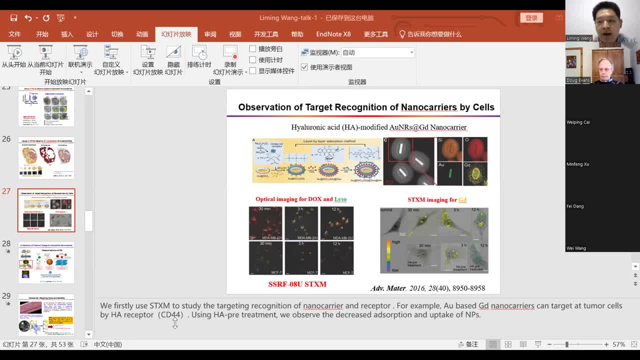 Lianfeng Zhao, PhD Chemical. Lianfeng Zhao, PhD, biochemical, with such as SPR and a proteomics. proteomics can be sure the director interaction. now we are doing the similar work. we found some material that can honey talk to this picture memory. we don't know what the kind of protein, so we can. 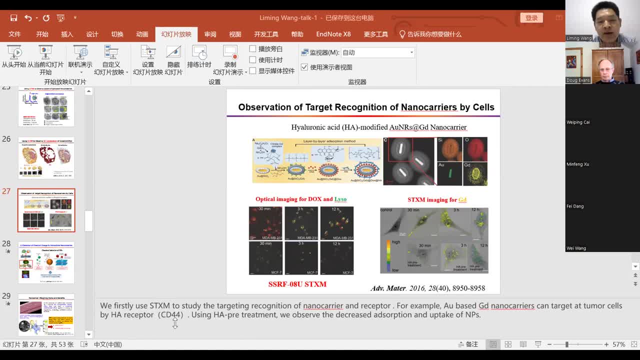 Lianfeng Zhao PhD, separate the cell wall or cell membrane back to your memory and back at your work proteins and and break them into Lianfeng Zhao PhD, into proteins. then incubated the, the. the protein interact with a particle to see what a kind of protein are enriched on surface the particle. if they leave first away, you can find that your target the protein. then you use the label- metal label- to to specific a protein. so I think of the proteomics and the x3. imagine they can be combined together to see how they interact with the particle. 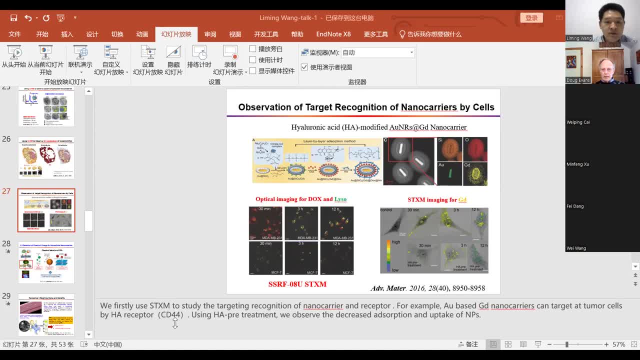 Lianfeng Zhao, PhD, With the proteins. Lianfeng Zhao PhD, So i'm not sure whether I did. this answer either can well address your concerns and prefer the poem Christopher Cameron Welton. Well, I would also remind people that you're more than welcome to get in touch with our speakers. 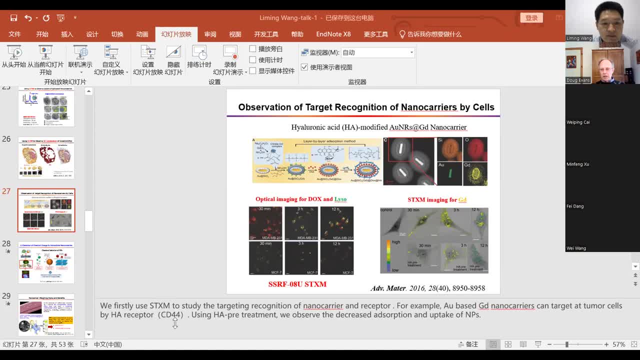 Christopher Cameron Welton, And if you need to get an email address, you can contact Julia colleague, who's our events coordinator, and she will put you in touch with speakers if you want to follow up on any of those questions, We have a question from Kelly Evans who asks: thank you for your talk. 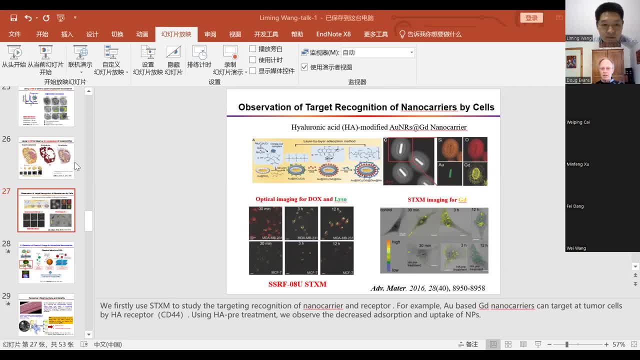 I'm wondering if nanoparticles are more likely to bind to proteins located outside the cell membrane compared to those located inside the membrane. Thank you for your question, Dr Evans. This is a very good question. I just answered to Dr Peng, I think. 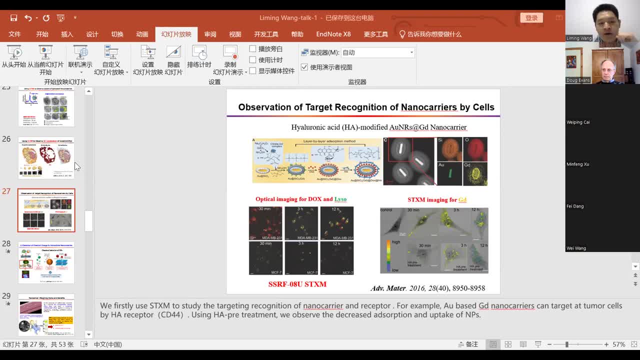 we need to use some biochemical tools to study which protein is better or has a stronger affinity to the nanomaterials. I think, for example, if we want to study the outside, the protein, we- just outside the membrane- we can. we can first detect the proteomics. 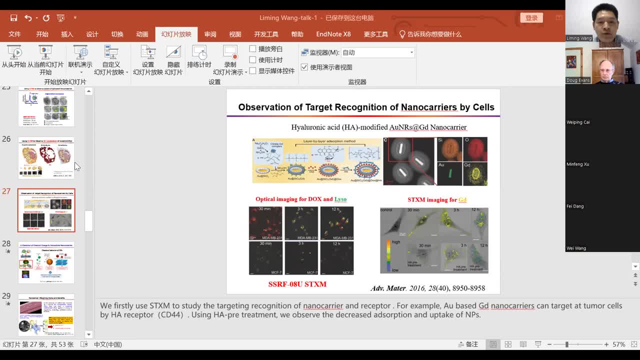 of the protein To detect what kind of protein prefer to absorb on the surface For the inside of the membrane. we can break cells into pieces and go to the cell nests of proteins. interact with the materials. We get another part of proteomics. 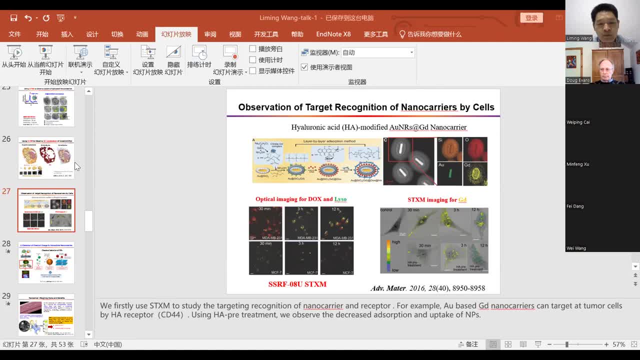 So from the two parts of proteomics we get different specific proteins. Then we use some methods like SPR and BLI and MST- other methods- to detect the binding affinities between nanomaterials and the different proteins. So that increases our know time. 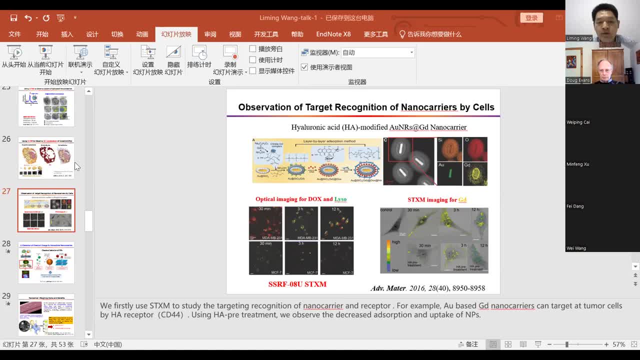 It also depends on the material type, also on the protein type. Sorry, Thank you, I'm not sure my answer can well address your concern. I think that answers the question. Okay, I think, given the time, we'll call a halt to the questions. 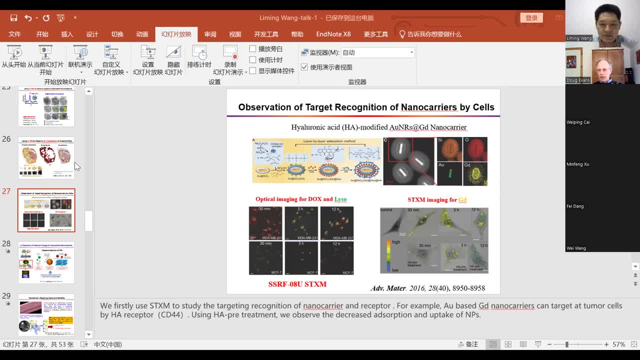 Again, as I said, you're more than welcome to get in touch with our speaker and ask additional questions by email after the talk. I also would remind you that these lectures are recorded, And so you can always go back and look at them from our website on our YouTube channel. 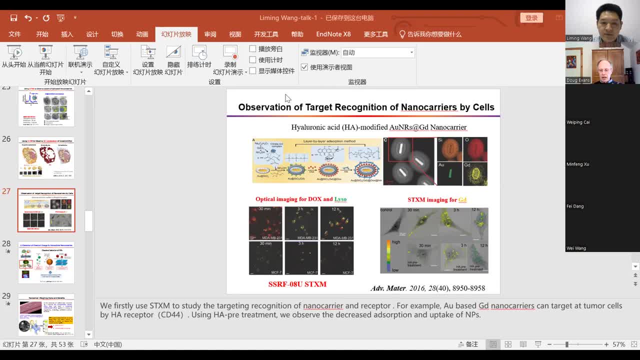 If you have any trouble getting access to the recorded talks, just get in touch with either myself or with Julia Colley and we'll find a way to make sure that you can see them. And I just want to give a bit of a preview of our talk for next week. 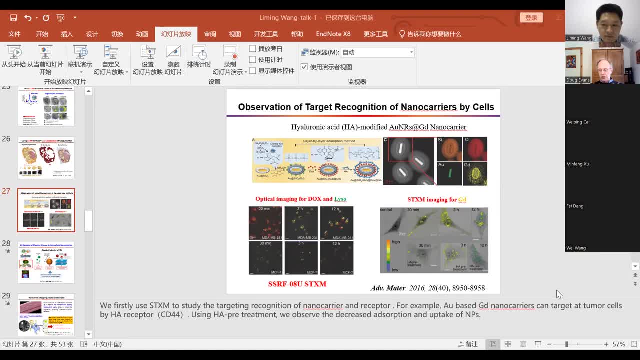 Next week we will have Jason White from the Connecticut Agricultural Experimental Station. We're going to change the nature of the talks, where we're going to get more into applications of nanoparticles, And Jason will be talking about nanoparticle-enabled agriculture next week. So I would invite you all to come back and hear that talk. 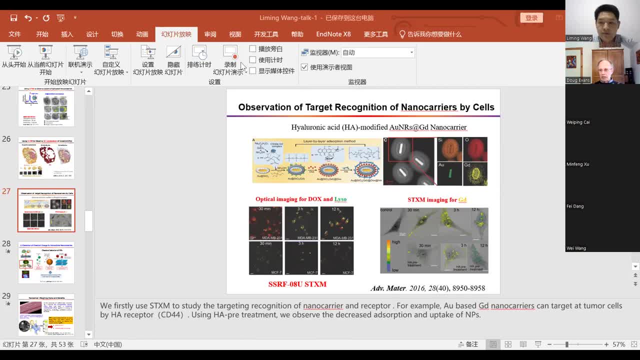 That will also be a very exciting talk, And I want to just conclude today by once again thanking you, Professor Wong, for this really interesting talk. We really appreciate you taking the time to speak with us, And you've certainly introduced an area that's going to be very important. 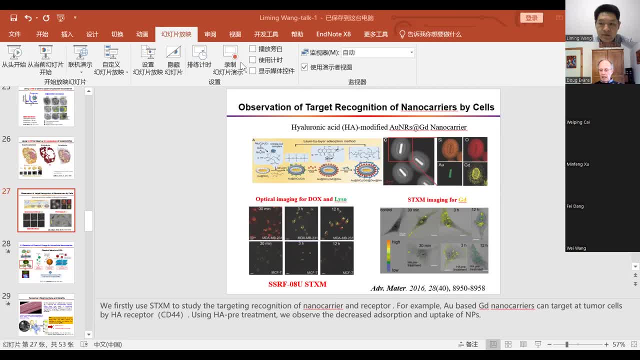 as we start to look at using nanoparticles in a lot of different biological systems. So thank you again for today And thank you all for being part of the lecture today. See you next week. Thank you, Professor Evans. Yeah, Bye for now. 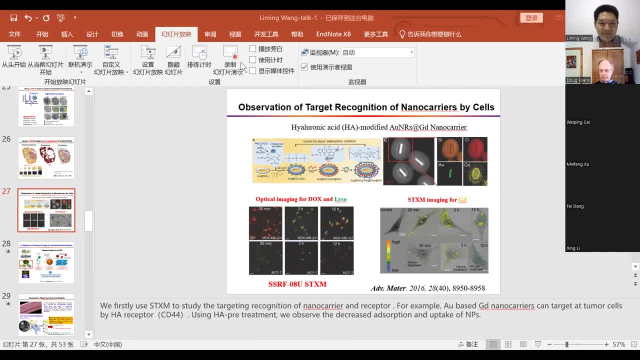 See you next time. Bye, Bye. 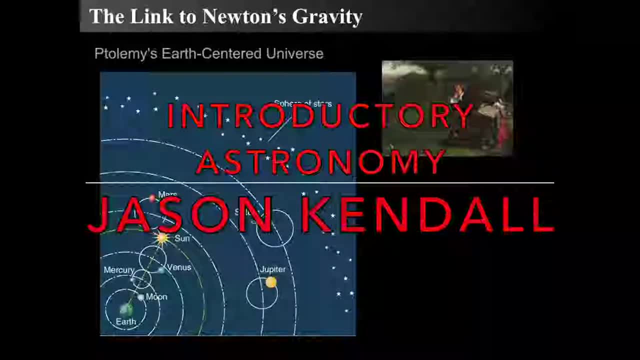 Hello, this is Jason Kendall. Welcome to the next of my introductory astronomy lectures. This time we're going to continue on our exploration of the Milky Way And we looked at the rotation of the Milky Way through the spiral arms. We saw that they were made up of stars and dust and gas. 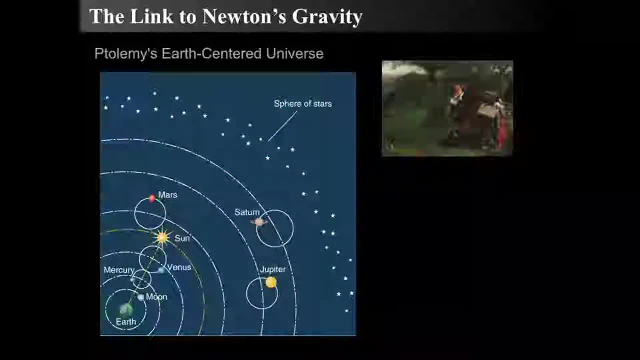 But there's something interesting. if we study deeper into the nature of the Milky Way, One of the things that you could ask is that: how fast is the Milky Way rotating? And that's a really good question. So let's actually begin really far back and go all the way back to Newton and the apple tree and the grand old thing. 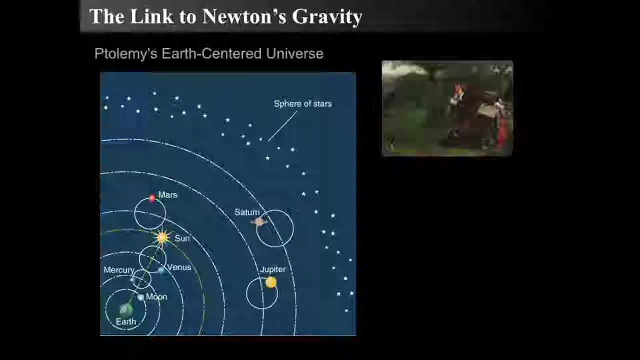 But let's go way, way back And remember the old thing where Ptolemy said that the Earth was at the center of the universe and the Earth was everywhere and all the stars and those things were orbiting in spheres and so forth. 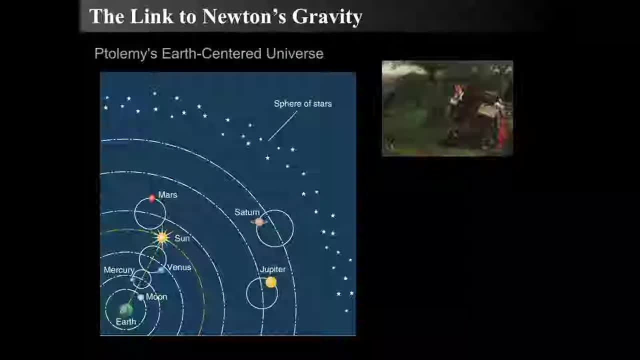 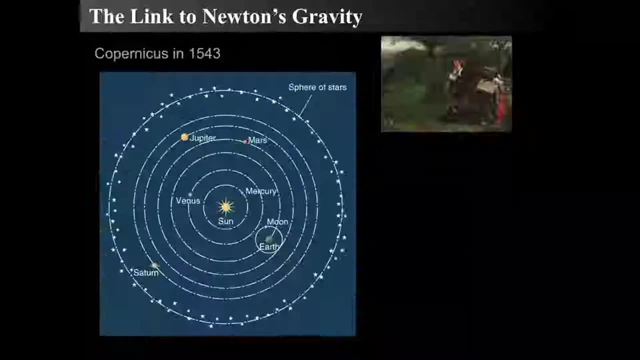 And people eventually discovered that that didn't work. Mr Galileo came along and showed that Venus had to be orbiting the sun and Mars's orbit could only be explained by elliptical orbits. And but Still though, Copernicus tried to place things in a new way in 1543, put the sun at the center, but still kept pretty much everything else the same. 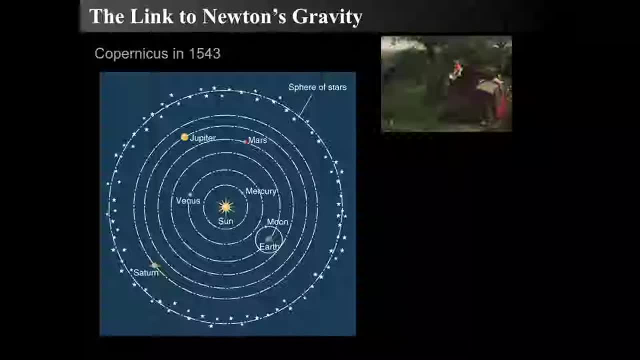 He did this posthumously so he wouldn't be hanged. So that was kind of an important thing. So Copernicus came up with this heliocentric idea, mostly because it was just easier to do in a certain sense. You got to admire that.